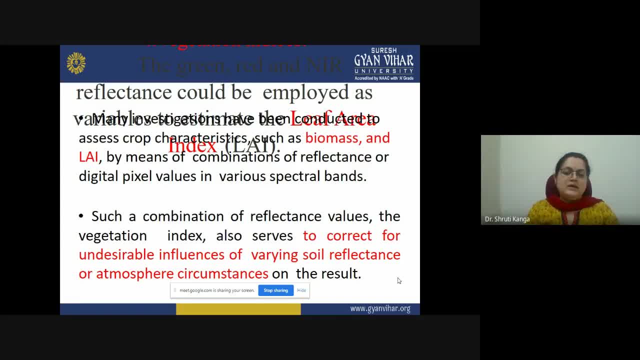 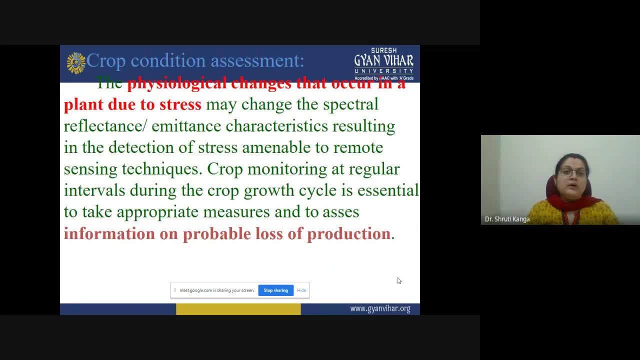 calculations. At the same time next, we will also discuss about the the生息, Ilia Ferrignano, citric acid companies and if, if, ambiguous again. At the same time next, we have discussed about climate action: Bettering Luqshan agriculture. terrorist sand-licking ceremony and so on and so on, For an example of different species and activities that the world is really focusing on. you have discussed about issues of environmental habitat conservation, artificial樂 Adding防, gospel to Bruckenheide, earthen fox, energ免ガalter and other Covid-19 conditions. 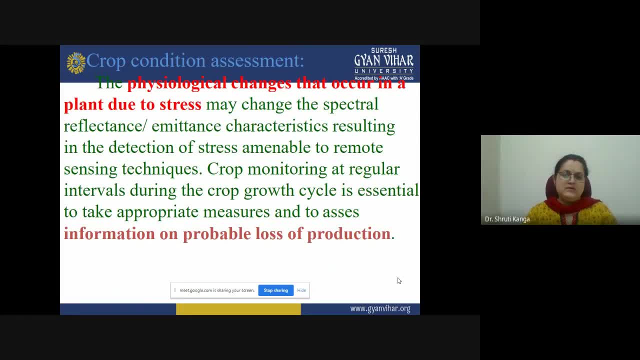 How is the problem proving Sweden's mushrooms about garbage arrest, some problem in the growth activities due to some infections or due to some- um you know- nutrients, lack of some nutrients? then they can be managed based on different uh physiological changes that occur in the plant due to different kinds of steps which may be recorded in the form. 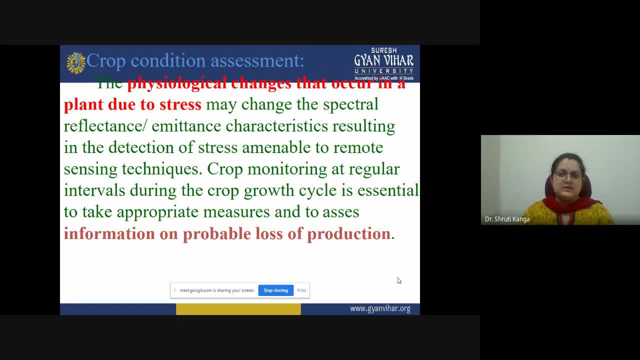 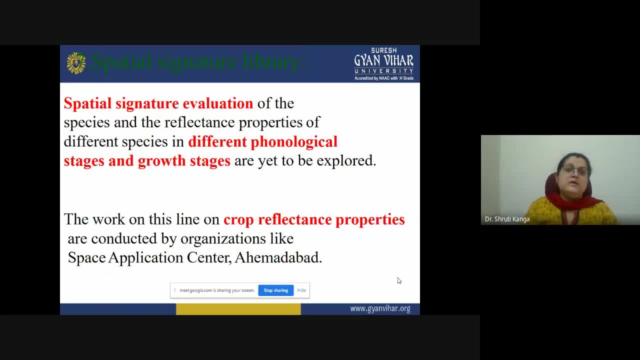 of their uh spectral reflectance or emittance characteristics, then phenological studies can also be done. uh, then the spatial signature library can be uh evaluated and then we can go for the different kinds of prop. uh, uh, you know uh stage and growth stages, exploration activities and 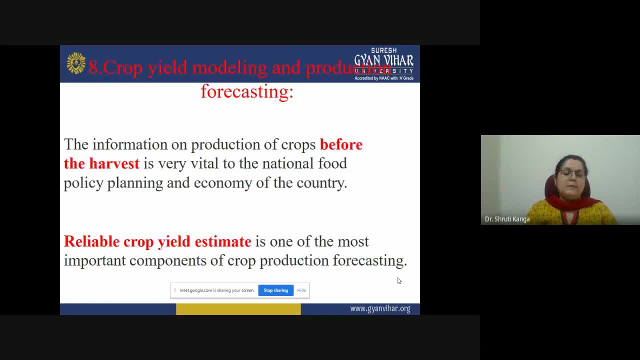 then we can go for or plan for different management strategies. then we can also um go for the crop yield modeling, where we can uh, on the one hand, we can assess about the yield uh, what yield we are uh about to get uh from the production of a particular 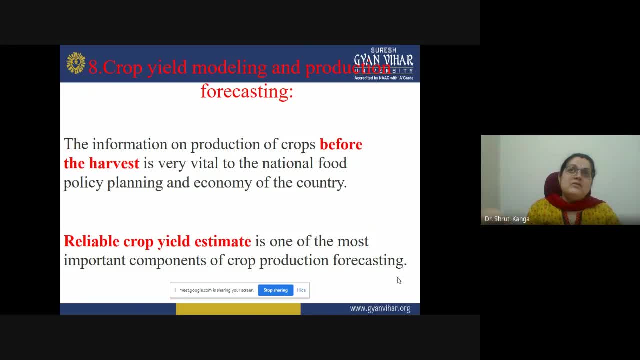 crop type and we can also go for the forecasting how uh the behavior of these uh productions can be in the future, so that we can, if there is any lacking of the production, then we can go for different uh strategic management so that there cannot be a, you know, insecurity of 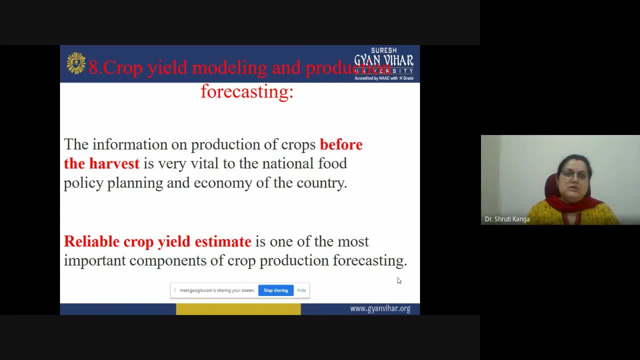 food in terms of the lack of production activities of a particular crop type. so this is really helpful in, you know, maintaining the price of the crops. uh, if there is a lack of a particular crop, so we we can in, uh, you know, advance, we can ask for the uh. 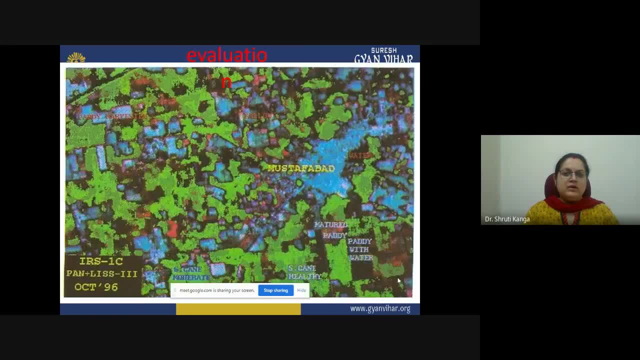 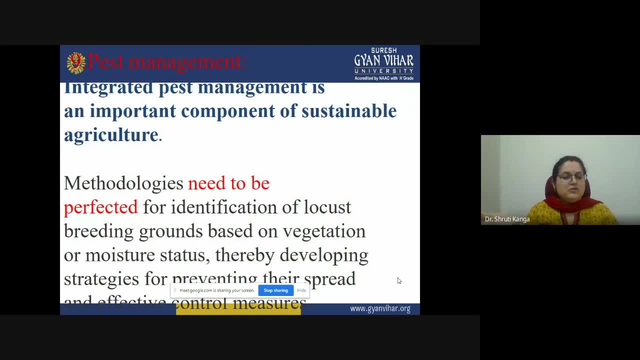 management of those activities. okay, then we have uh the next application, that is, pest management. okay, because uh, on the basis of different reflectance values, we can uh have an idea about the uh- you know, different kinds of um infections where the pest infection is one of the uh cause. 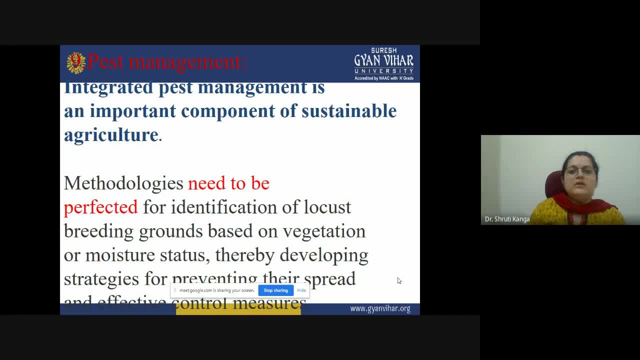 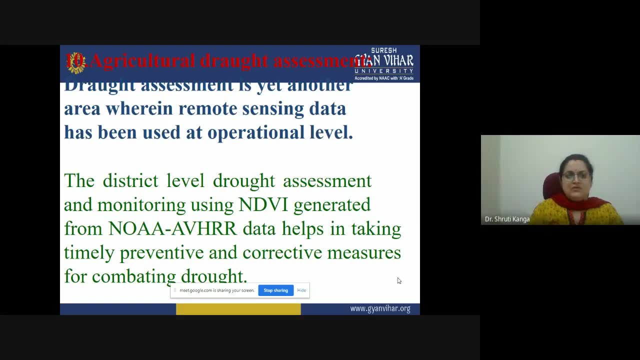 due to which there is a loss of- uh, you know, different crops. so for those kind of management activities, then here we have left. in yesterday's class we were just revising what applications we have studied in yesterday's class. now we'll start with the agriculture dot assessment. now we can also go for the broad assessment. uh, this is another application. 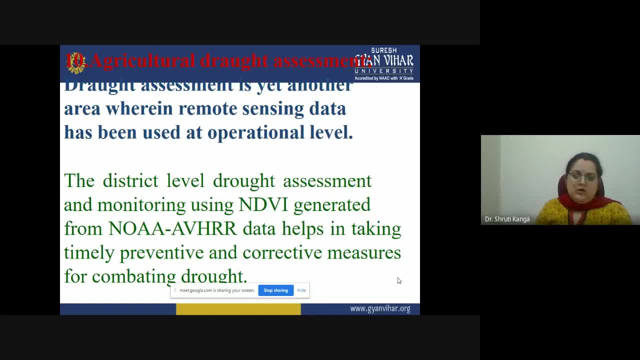 of uh remote sensing, uh scope or, if you can say, geospatial tools which can be used for the agriculture drought assessment activities? uh, how we can go for uh you know different levels of uh drought assessment and monitoring using different uh techniques which are related to maybe. 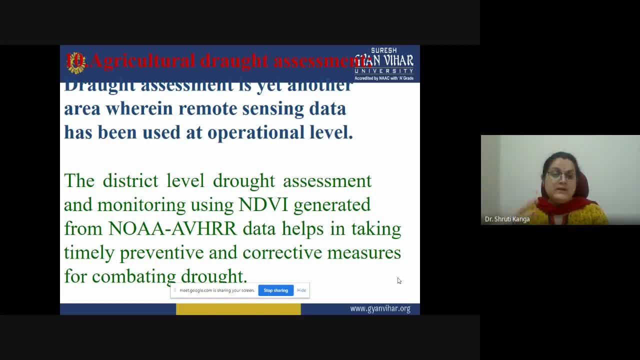 ndvi, where we come to know about the density based on uh, the or the health of the uh. you know the, the different crops on uh, so we can go for the change detection also if the production is regularly decreasing, decreasing and decreasing. so some time will come when the production will be uh zero for a particular uh you know uh crop or for different. 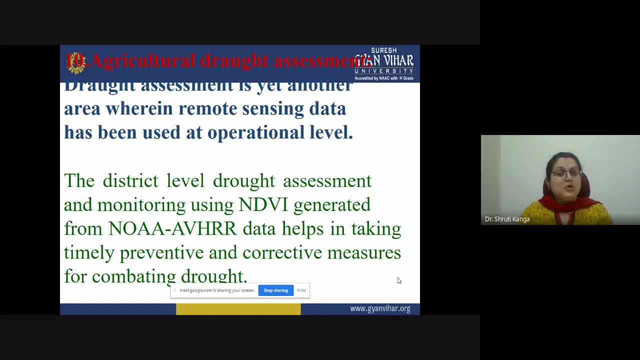 agriculture product in a particular area. this may be cause of uh, some hydrological parameters, that may be some because of some uh metallurgical parameters, or it may be some due to some you know parameters which are there, existing uh. so we need to observe those parameters, uh for that particular area. and 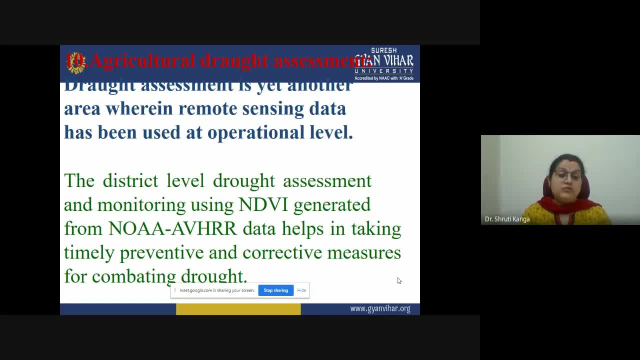 then we can go for different preventive and corrective measures for, uh you know um combating different droughts, like metallurgical droughts. if we are talking about that, there are, uh you know, uh, because of lacking of uh, water or moisture content in the um area, uh the drought like conditions are appearing. then we need to take care about the different. 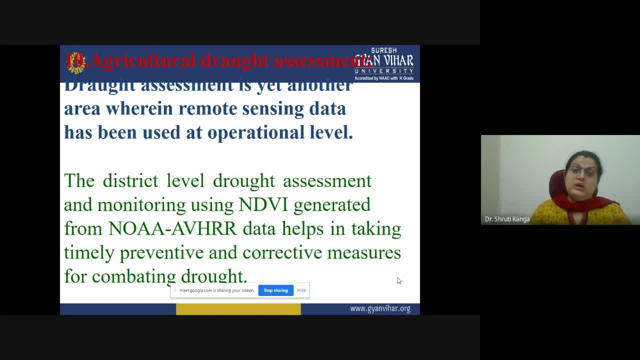 hydrological parameters in that areas. we have to maintain those kind of things. we have to go for maybe the water potential site zonation mapping, or maybe the water- uh, you know, watershed management into those areas. those kind activity, kind of activities we need to, uh, you know. 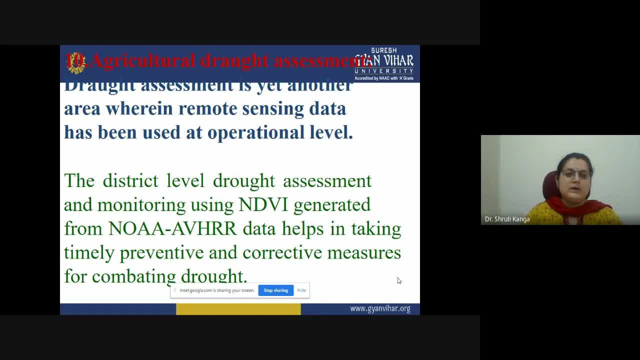 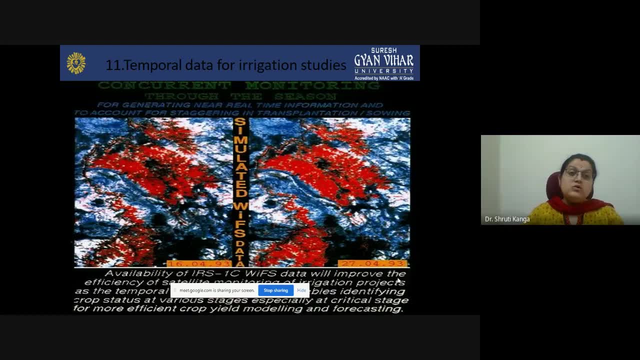 in that area to manage or combat the drought-like conditions. then we have the temporal data for irrigation studies. okay, we can also have studies like: irrigation is a major- uh, please, major- role in any kind of- uh, you know uh- activities related to the agriculture or other vegetation related activities. so, um, if we know that especially, 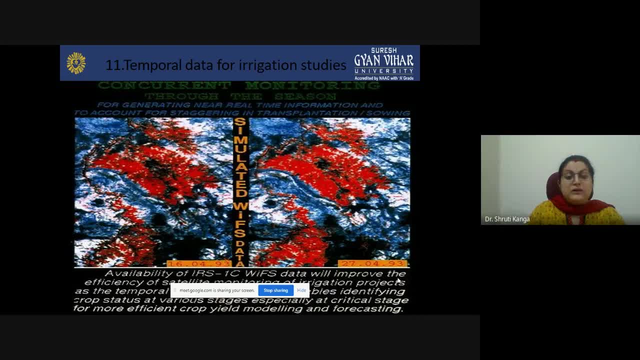 related to각ugar uh days, like in uh dry states like rajasthan, madhab, даish uh or many other states which are having uh droughts in uh particular season. okay, so, because of the hydrological or climatic conditions. so, based on the uh, you know, multi-temporal data of a year of 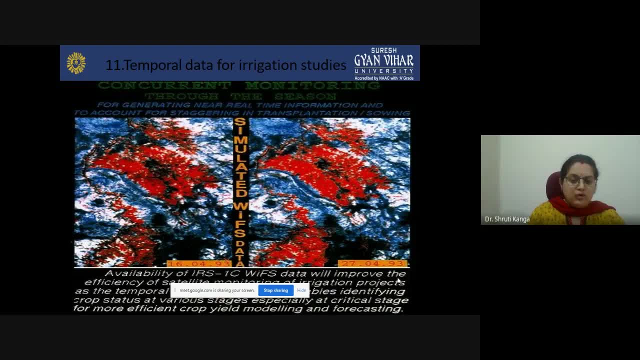 different seasons, we can see the pattern of- uh you know uh- activities in which season we are using the natural sources, in which season we are using the artificial season, or, if there is an excessive rainfall, how we can store those waters, which is related to water harvesting or watershed management. related activities can be performed. 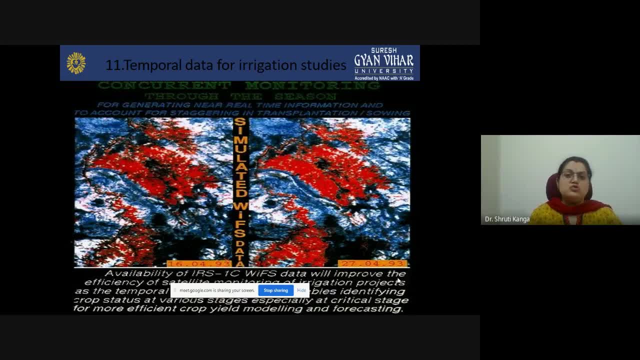 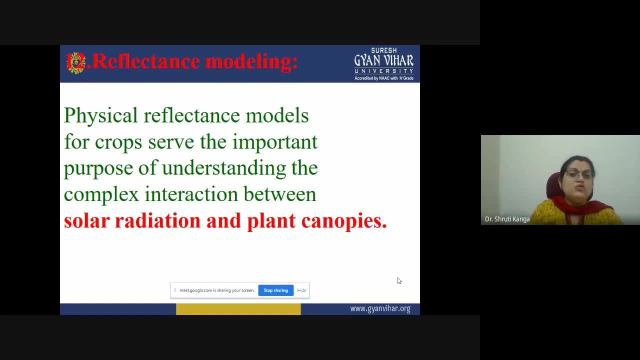 So different kinds of temporal data can be used for different kinds of irrigation related studies. Then we can also go for reflectance modeling, where the physical reflectance models for crop serve the important purpose of understanding the complex interaction between solar radiation and the plant formation- canopies. 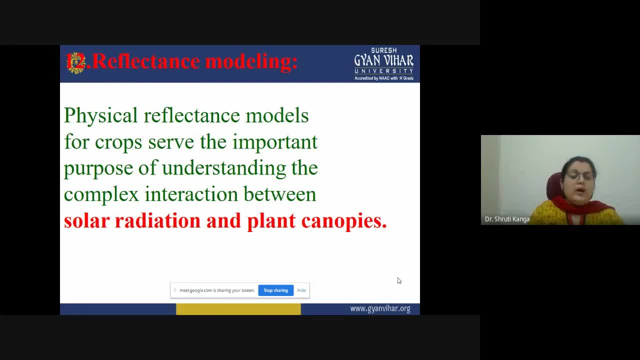 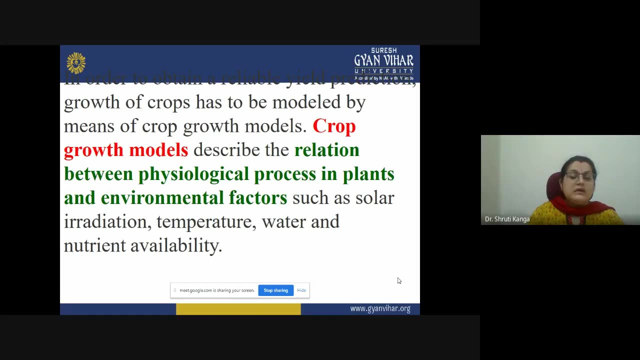 So, based on the various reflectance values and their interaction between the solar radiation and plant canopies can be done. So related studies can be done. So the reflectance values of different crops can be used for different kinds of crop growth models, which we have studied in the previous application where we were talking about the 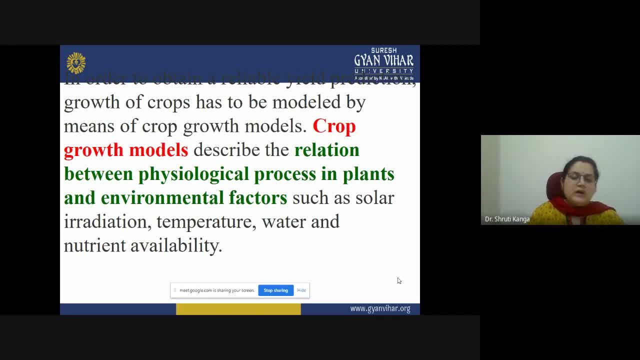 growth rate or the production of the different crops can be managed. So, in order to obtain the reliable yield, production growth of the crops has modeled by the mean of crop growth. So crop growth models describes basically the relation of physiological processes in the plant and the environmental factors such as solar irradiations, temperature, water. 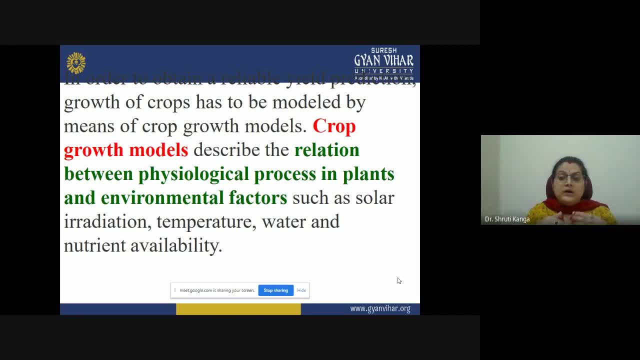 and nutrient availability. So when we are talking about crop growth models, they can be applied. when there is some relation in the physiological process, Okay. And the environment factors, like environmental factors, like the- you know, health of the soil in that particular area, water, humidity, temperature, all these things, along with the 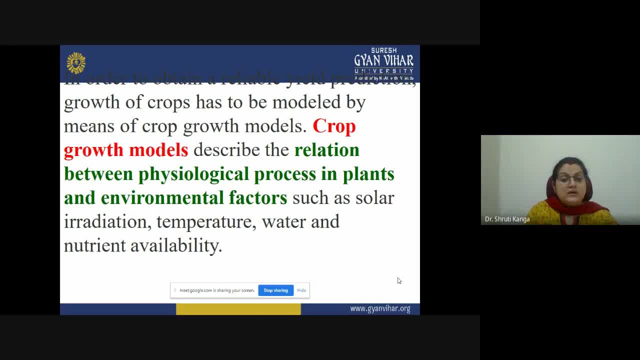 you know, species or type or different physiological processes Are in collaboration. So, Okay, Okay, Okay, Thank you, Thank you very much, Thank you, Thank you. they can uh have a, you know, idea about the growth models of various crop crops. 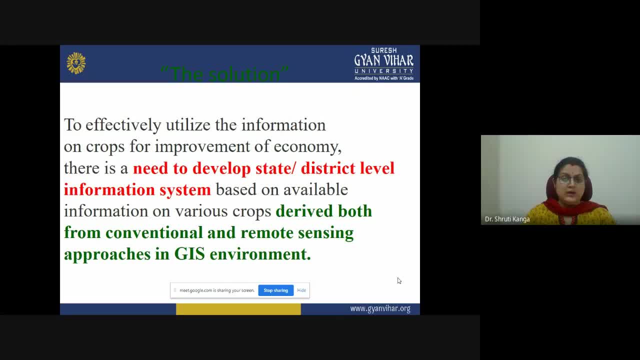 then the solution: okay, so what? what can be the solution for the improvement of, uh, you know different crops so that we can uh directly or indirectly improve the economy of that particular place? so, to effectively utilize the information on the crops for the improvement of economy, there is a need to develop a state or district level information system based on the information. 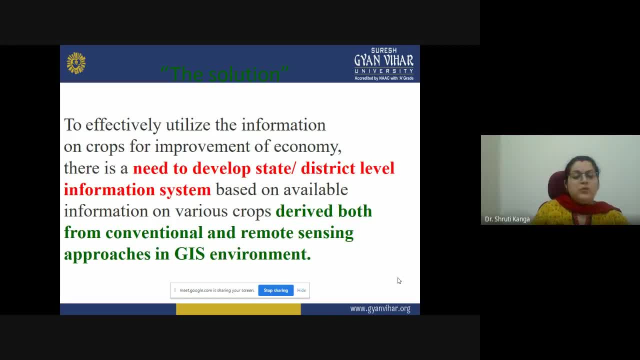 of various crops, derived both from the conventional and remote sensing approaches in the environment. okay, so what is the solution? how we can, uh, you know, apply, uh, all these applications which we have discussed in today's and yesterday's lecture. we have to, uh, you know, uh, uh, we have to apply different kinds of conventional techniques. 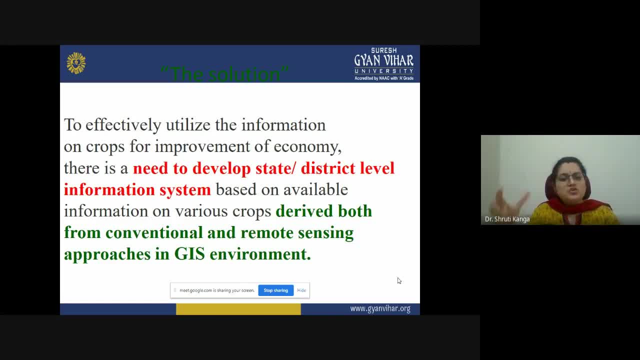 in collaboration with the uh different geospatial technologies. uh to uh have an idea about the you know different crops. it's at different levels. it may be village level, district level, state level at as a nation. in whole, okay for the improvement of the crops as the uh you know uh our economy is. 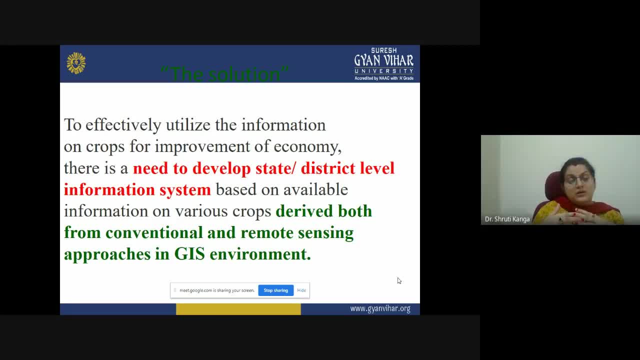 based on uh the forest and the uh you know agriculture. so we need to go for a regular and continuous studies which are based on not only the conventional data which we are having about the uh you know particular area, about agriculture or different land uses, but we need to collaborate different uh remote sensing applications. 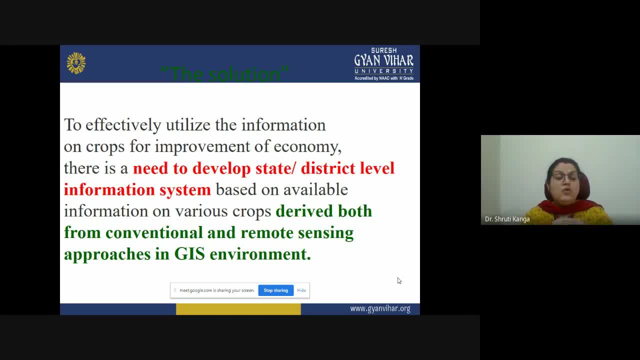 because they uh go for a you know uh synoptic view of a particular area in a single go. so uh and gis, it helps in the collaboration of your local 那樣楣. welfare these conventional and remote sensing based data sets in a single platform where we can correlate. 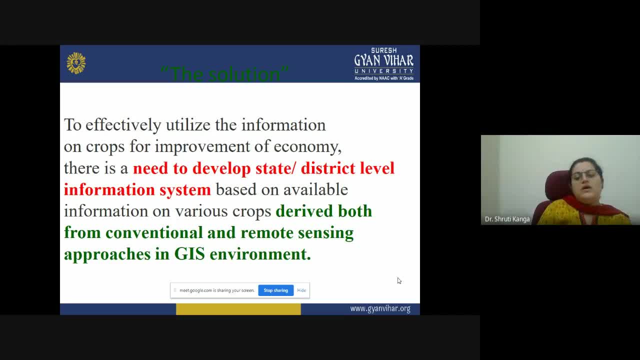 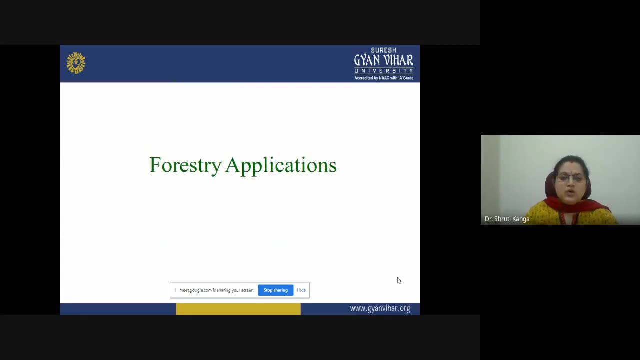 all these things and we can utilize it in better manner. uh, for improvement of the, you know, various economy at various levels: at at village level, at state level, at district level, at block level or the sea level. okay, so this is the solution. this is means remote sensing, gis and the conventional data. 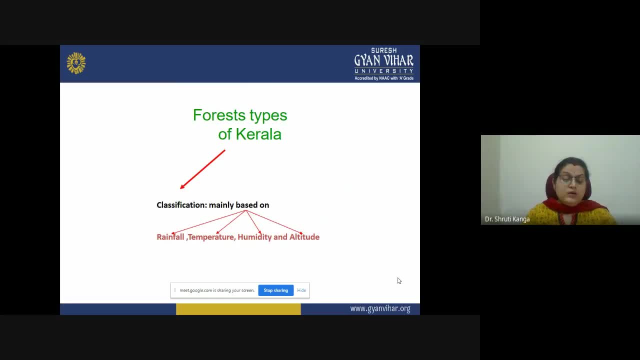 integration now uh for showing uh different applications of, uh you know, remote sensing and gis. we have taken a case study of an eduki district of kerala, where the forest types of kerala uh first categorized and then the classification uh was, uh you know, done on the basis of rainfall. 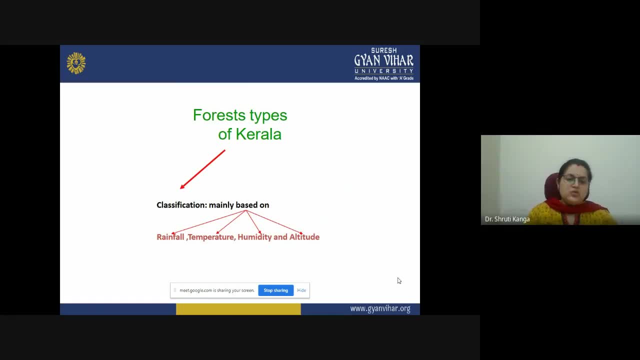 temperature, humidity and altitude. okay, so uh, for forest applications. firstly, the case study which we are taking up there. they have, uh, you know, done the classification of forest types in a particular district of kerala, where the main basis or the main factors which they have taken for the cons, 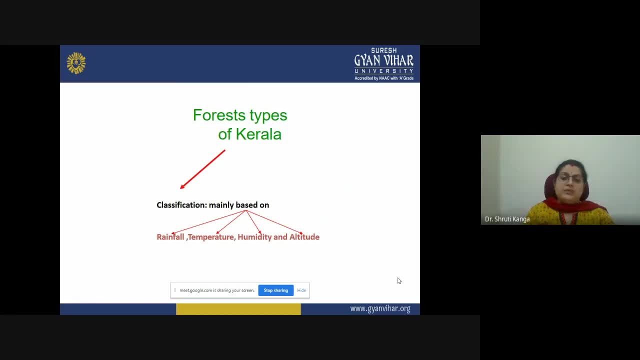 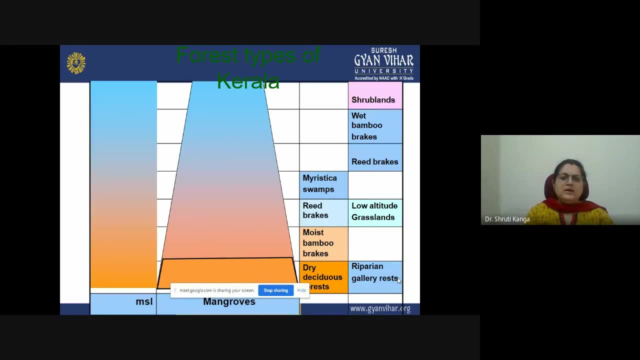 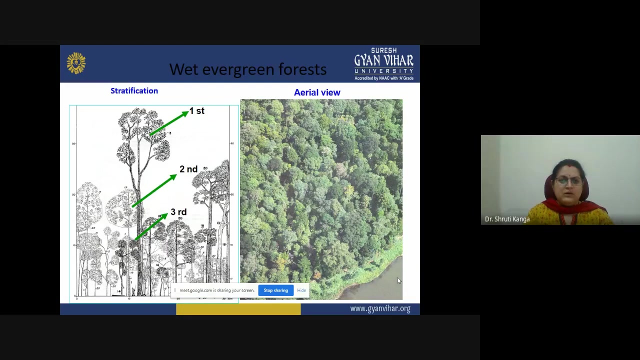 classification of forest was rain for humidity, temperature and altitude. so, according to that case study, the uh kerala is having uh these kind of uh you know uh forest types, where we have uh these many types of forests now, uh, this is the you know wet, evergreen forest and this is the aerial view of this forest. and 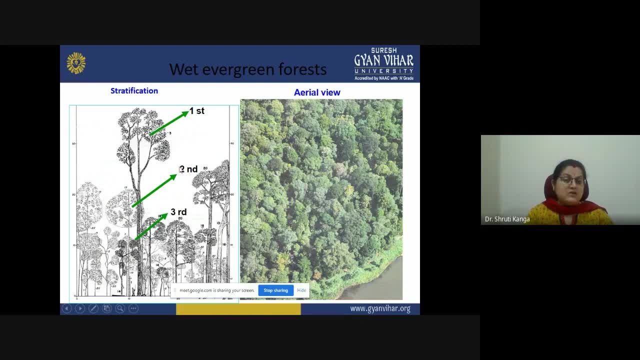 we can also have a studies of the stratification, as in the previous lectures I have told you that stratification is related to the ages of the tree. here you can categorize these trees. they have given number or to each and every tree and they have classed it into the three different ages. you know. 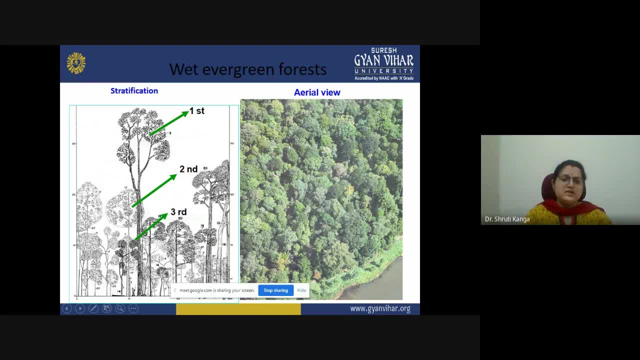 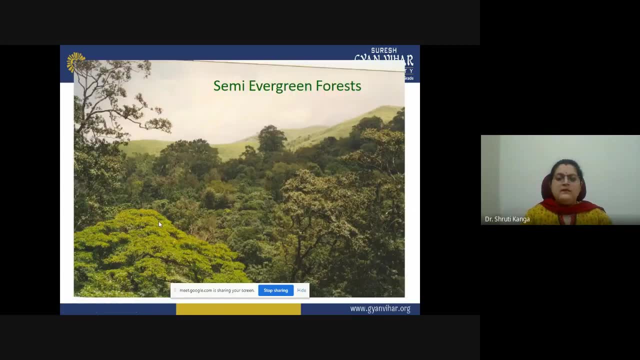 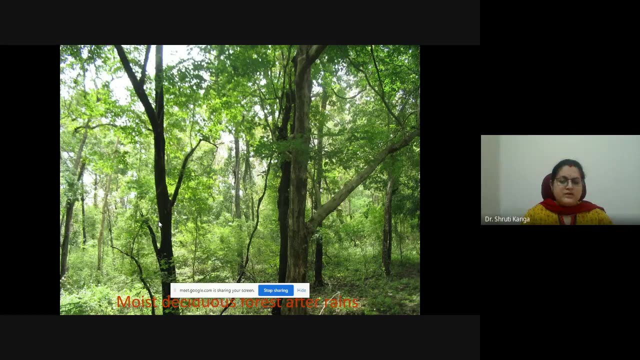 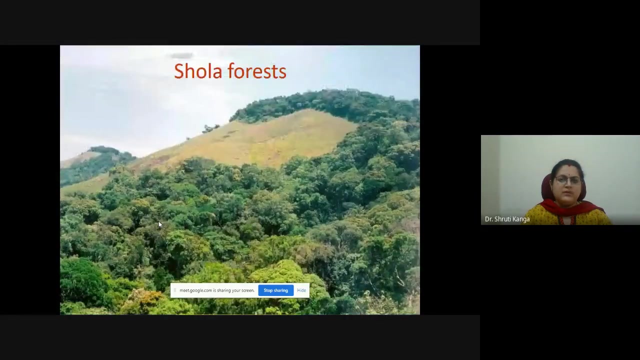 trees. you can see this is a first class, this is a second class and this is a third class. then this is a type of semi-evergreen forest, which was there in the Kerala, and then this is a type of moist, deciduous forest, okay, after rains. these are the grasslands, this is some chola forest now. this is 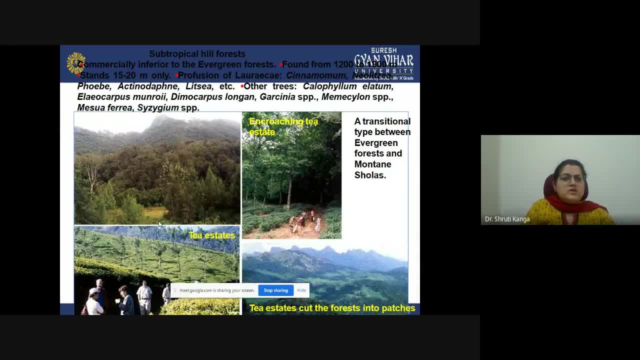 a subtropical, his hill forest, commercially inferior to evergreen forest. they generally found in the heights of 1200 meters to 1900 meters. the height of the stands it generally occurs in between 15 to 20 meters. okay then, the major types of forests are, or the products which are there. 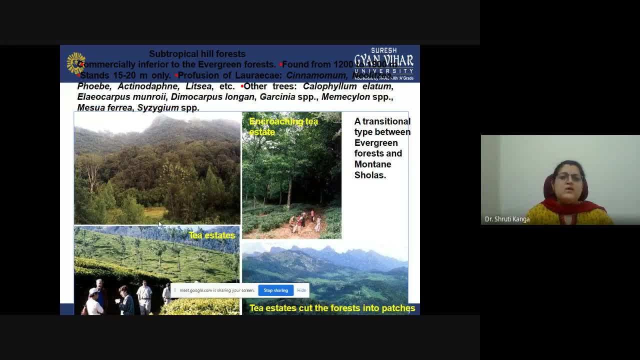 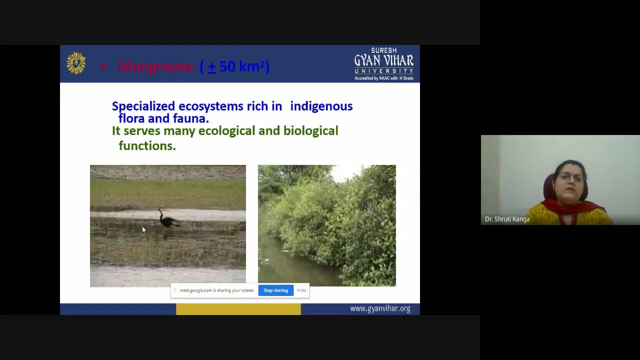 in the forests is cinnamon, neutral, Alesia, phobia, antiphoney, litesa, etc. other trees are these, so a transition type between evergreen forests to the mountain chola forest, so all the forest you can see in a single slide. in case of this case studies which we have taken up, then the mangroves plus minus 50 square. 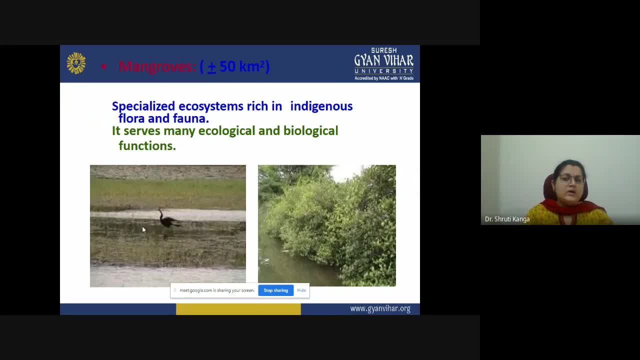 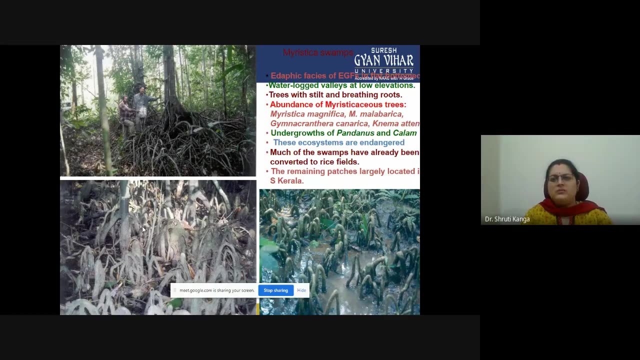 kilometers apply of climate row are with the saygies that are in the forest- we hear these- the specialized ecosystem, rich in indigenous flora and fauna, and it serves many ecological and biological functions. okay, then we have a swampy, edific faces of EFS, flat bottoms, water. 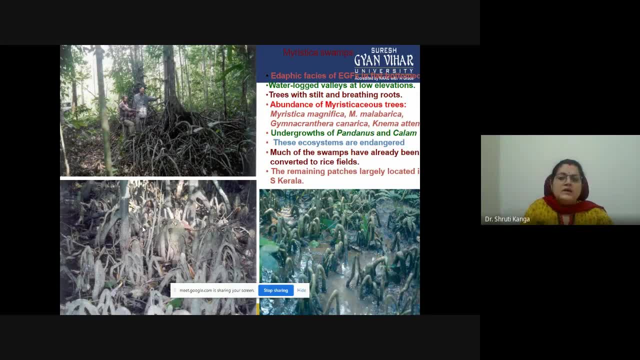 log valleys as low elevations. the tree is still stilt and breeding roots. abundance of this tree type my speakers trees, and then the under growths of column and the pendant pandanus. okay, these ecosystems are endangered ecosystems. much of the swampy have already been converted into the rice fields and the remaining patches are largely located in the 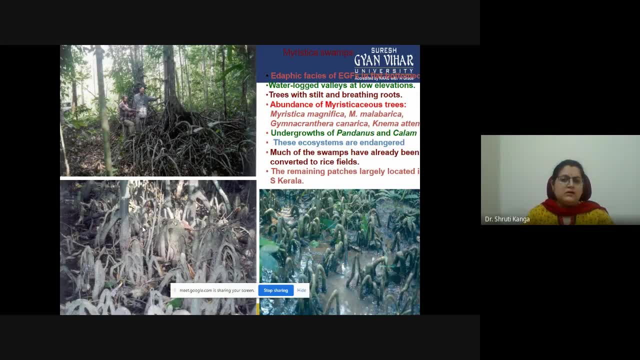 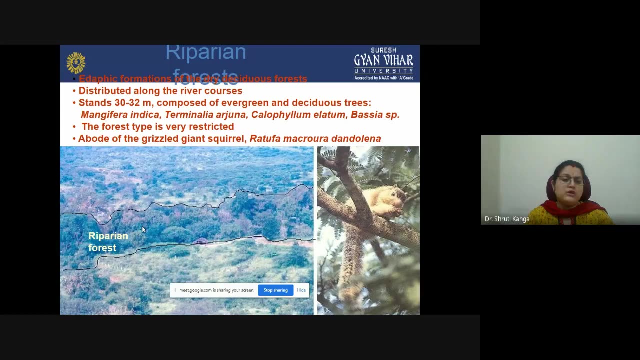 Kerala. okay, so this is another uh, forest type, okay, which is related to the swampy forest, and this is the characteristics which I have just narrated and you can see here in the photographs how it looks like. then riparian forest also found there, then edific foundations of the dry, deciduous 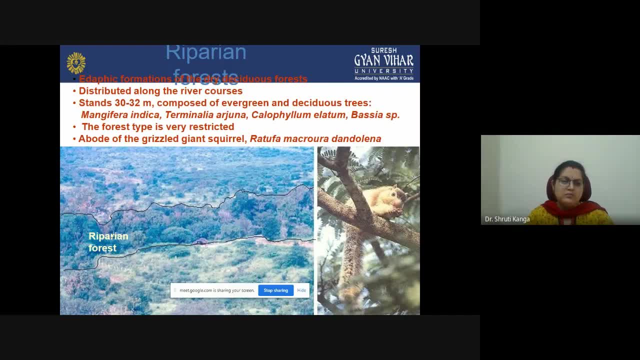 forest, which is also found there, then edific foundations of the dry deciduous forest, which is also found there, then edific foundations of the dry deciduous forest, which is also found there, then, and it composed of evergreen and deciduous, both the tree type, forest types. the forest type is 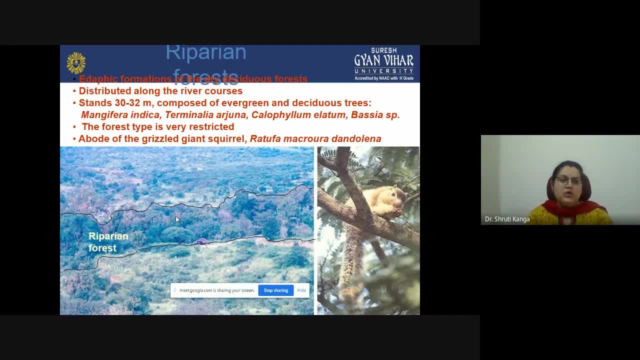 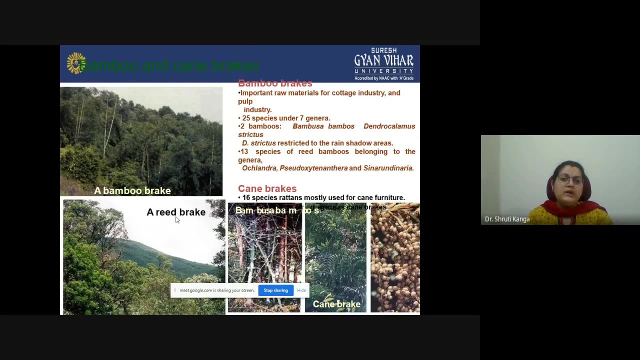 very restricted and uh abode of the grizzle giant squirrel and raptufa mycora. All these kind of fauna also can be found in this riparian forest. Then the bamboo and the cane brakes. Okay, Then, bamboo and cane brakes. 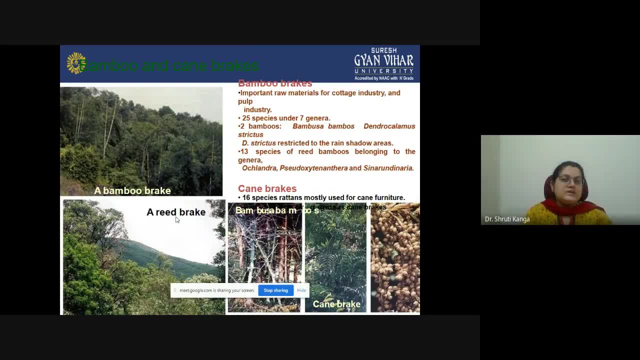 This is important raw material for cottage interest and pulp. Okay, This is again a type of forest which is found there, in which case study we have taken up. Okay, So bamboo barks and cane brakes. So this is the bamboo barks are the raw material for various cottage interest and pulp industry. 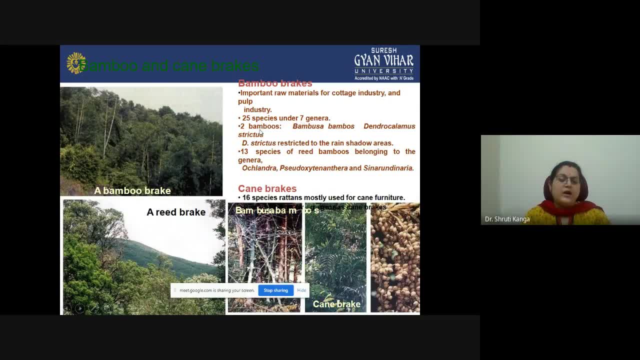 25 species under 7 generations and 2 bamboo species. Okay, Then the strictest restrictive rain shadow areas are there, Then species of reed bamboos belonging to the genus, And then the cane brakes have 16 species, mostly used for the cane furnitures. 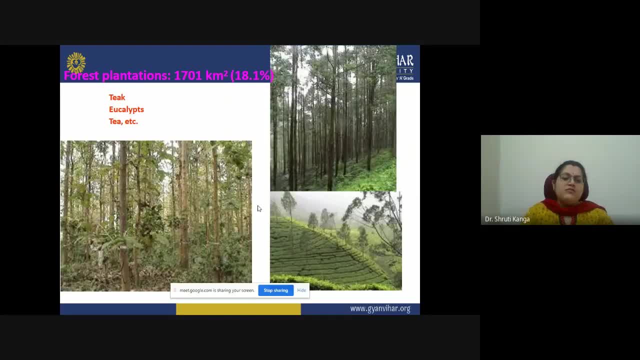 Okay, Then we have forest plantations around in 1701 square kilometer, which is of around 18.1% of total, for you know geographic areas. The major plant, The main types, are tea, eucalyptus and teak in these forest plantations. 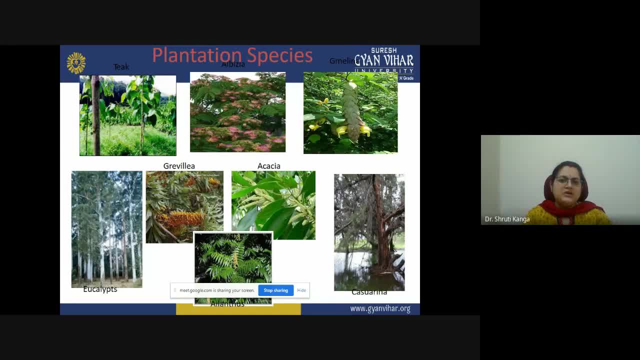 These are also there in the Kerala. Then plant plantation species: teak, abyssea, all these types of axia, eucalyptus. Okay, So all these are the plantations which are being done in these areas. 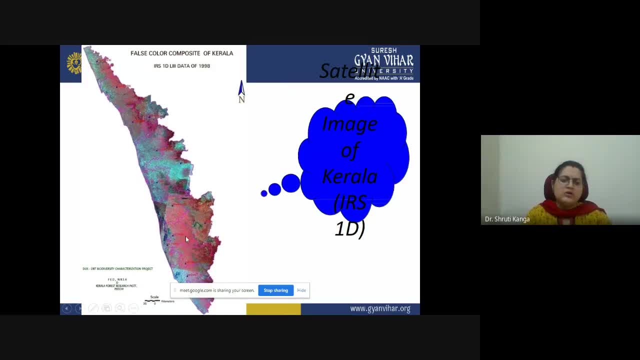 Now, if you see the forest color composition or the satellite image which is having IRS, uh, one deal is three data of 1998 in this case study. Okay, So here you can see complete Kerala, uh, as a satellite image of IRS one B. 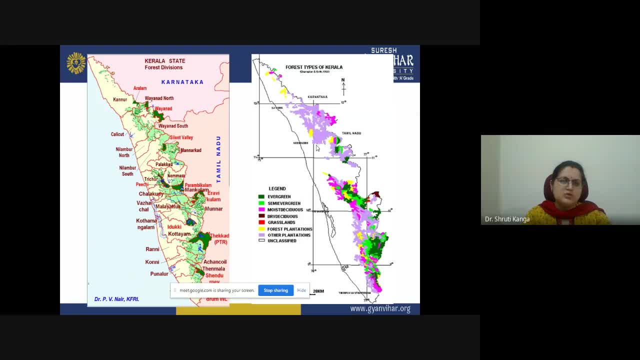 Now, uh, this is the different forest divisions. You can see the distribution. the red uh lines are denoting for different forest divisions of the uh, Kerala. Okay, Can you call it? Uh, okay, What's the first one. 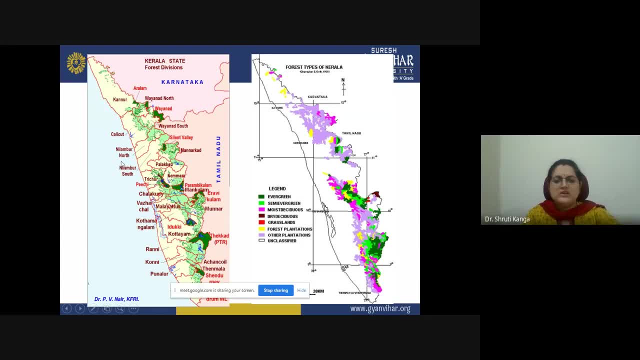 Nilambur, Okay, North. So these many forest regions are there in uh Kerala state Okay And the uh another map you can see the forest types of Kerala: evergreen, Semi evergreen, moisture, deciduous, Right. 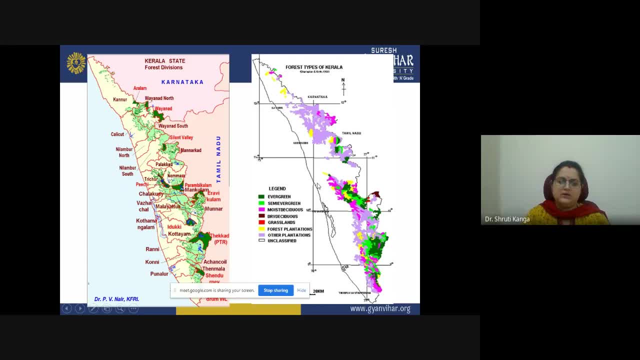 So the way we have tried, uh in uh through this, uh, you know, case study, Uh, uh, the different forest types which the author has taken. uh for uh for the uh for the different forest types. 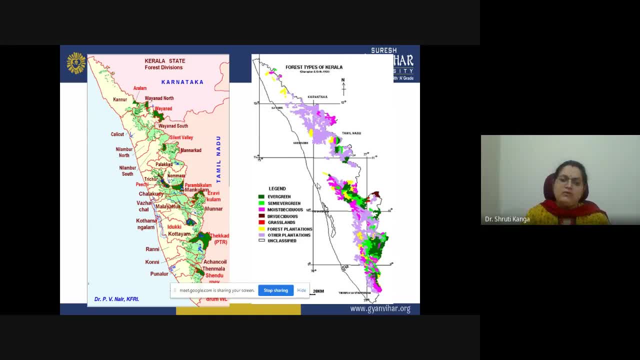 for the different forest types which the author has taken. Uh for the different forest types which the author has taken, uh for the uh for the different forest types for the classification. So this is how, if we suppose we want, 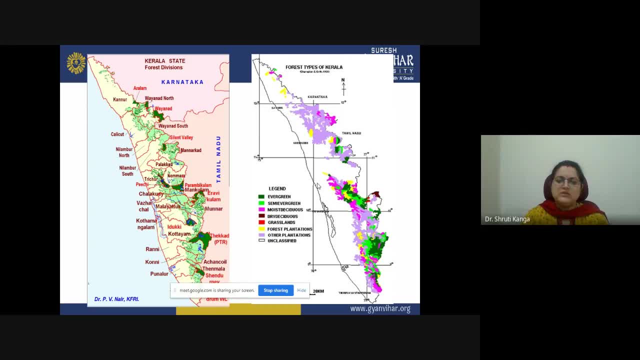 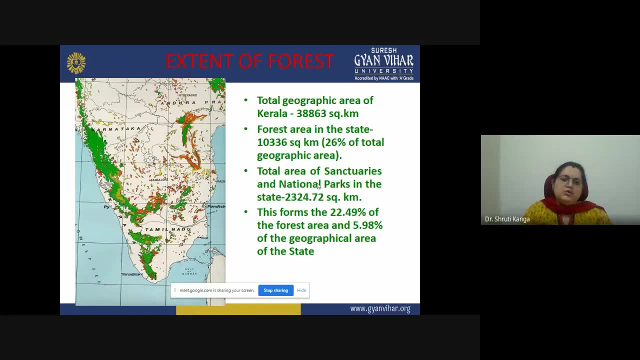 to go for some forest management activities. we have to also perform all these things. Now, the extent of forest in this case study, The total geographic area of the state is around 38,863 square kilometer, the geographic area- And out of that the state is having around 10,336 square. 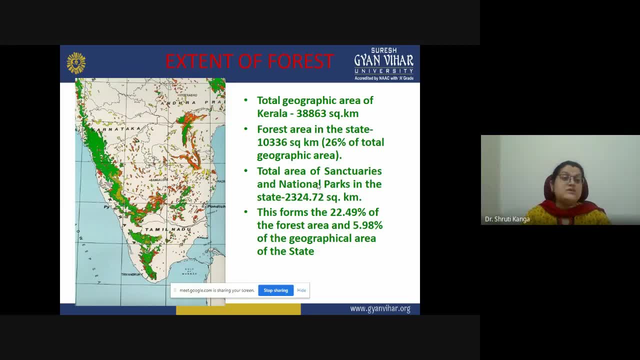 kilometer area as a forested area, which is around 26% of the total area of the complete Kerala state. Then the total area of sanctuaries and national park. we have a lot many parks and sanctuaries are. there is around 2,324 square kilometer area. 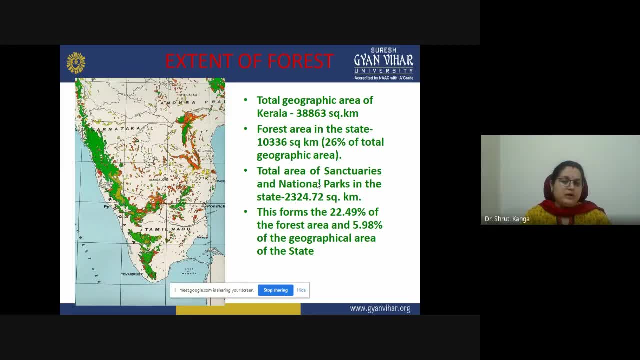 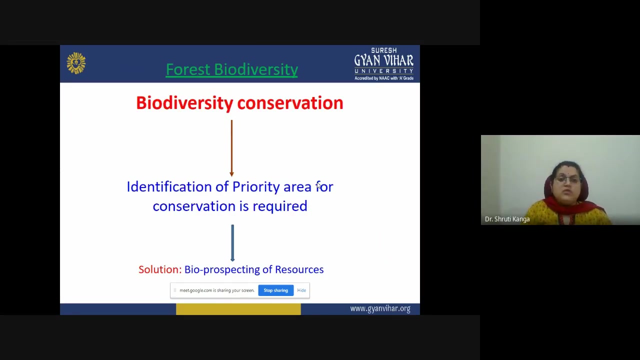 Then the forms of 22.49 of the forest area and 5.98 of the geographic area is a state, So the area it is having this many classifications of different forests or the land use types. Now the forest diversity. if you talk about the diversity, 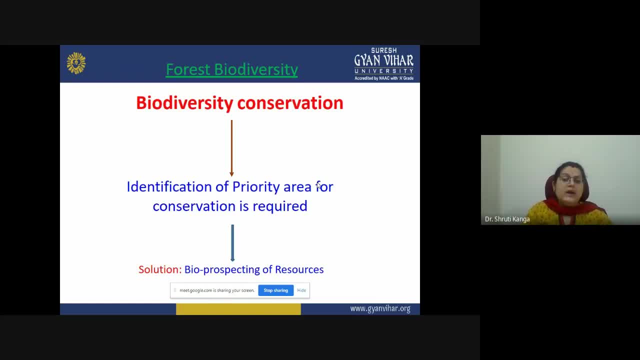 conservation- identification of priority areas for conservation is required- and then the solution- bioprocessing of the resources. So how they go for forest biodiversity, where they have to first go for the identification of priority areas which need conservation at the first stage. 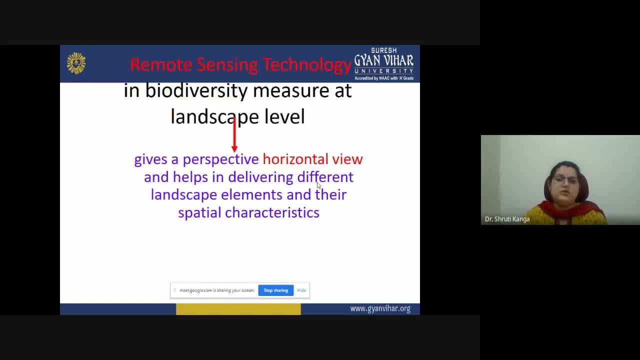 And then the solutions, how we can proceed for these biodiversity activities related to the management of biodiversity. So we are talking about two different bio-diversity. So remote sensing technology, how this is being used in biodiversity measure at landscape level, as it gives a perspective or a horizontal view. 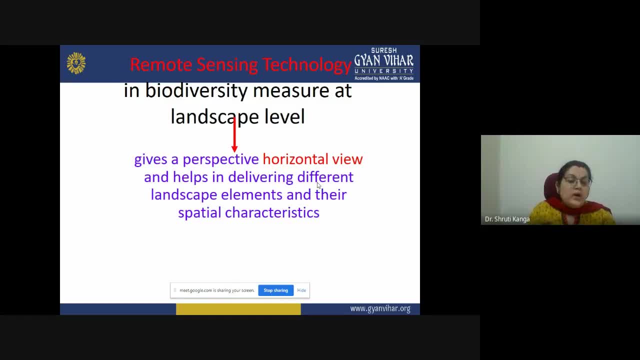 It gives us a synoptic view And also helping different landscape elements and their spatial characteristics. So what we can do, we can have a synoptic view in one go and we can also go for the identification of different landscape in a satellite image. 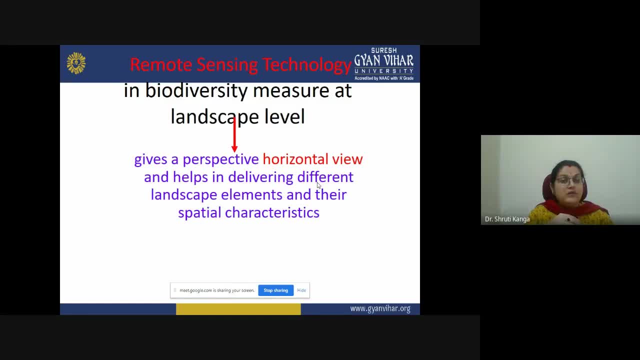 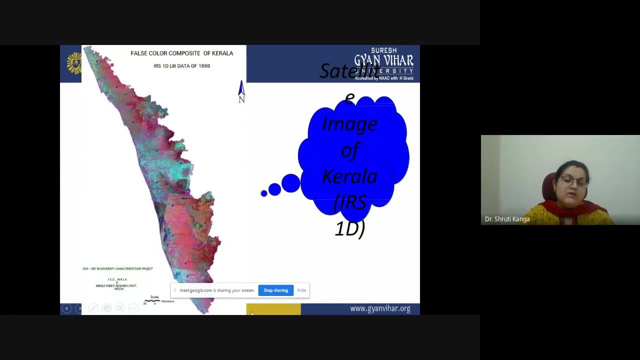 of the state in a one go where every feature have its own spatial characteristics. on the basis of what we can identify that what it is. If you see this sheet, you will find here different, you know- patterns, structures, color, symbology in this FCC. okay, so we can see that there is some maroon like color which may be denoted. 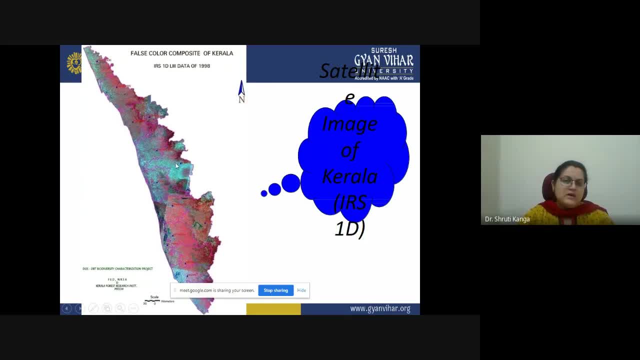 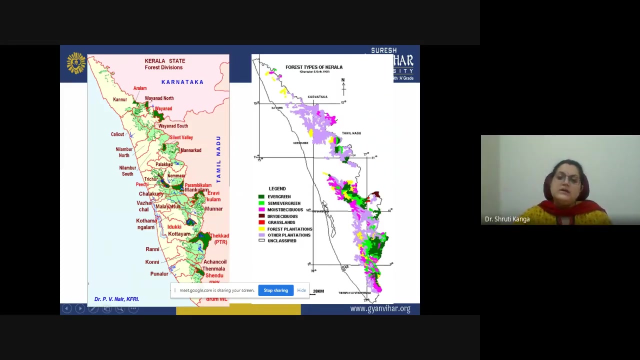 for some vegetation related activities. there are some. road networks are there, some, you know, water bodies are there, River some settlements are there, some waterlogged areas are there. So we have tried to identify different forest types and the part which you are able to see in the white, this is a non-forest area. 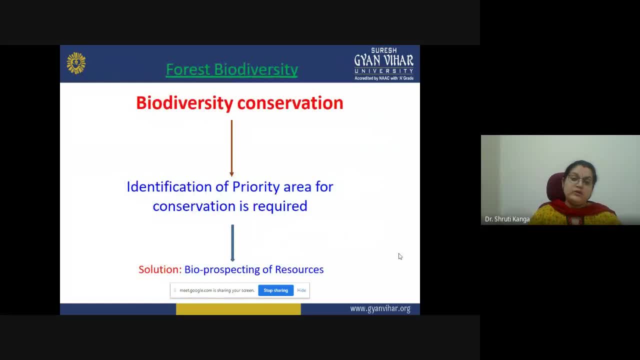 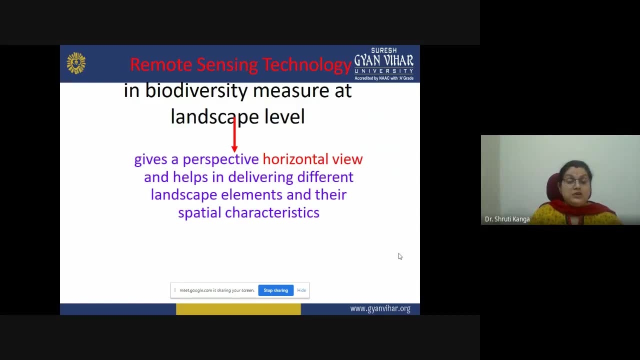 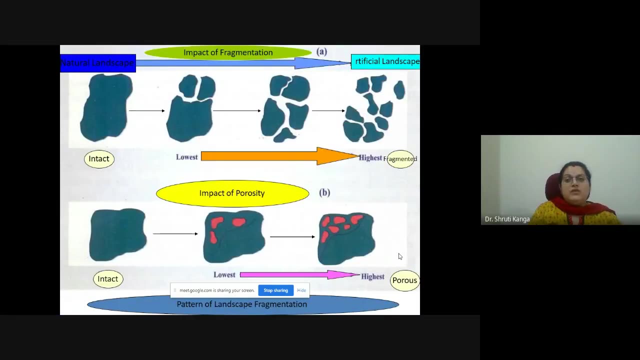 So how we are able to do it in one go, because we are using these remote sensing satellite data sets, which provides us a synoptic view in a single go. Then the impact of fragmentation. What is the impact of fragmentation means we have a bigger patch and, with time, the because. 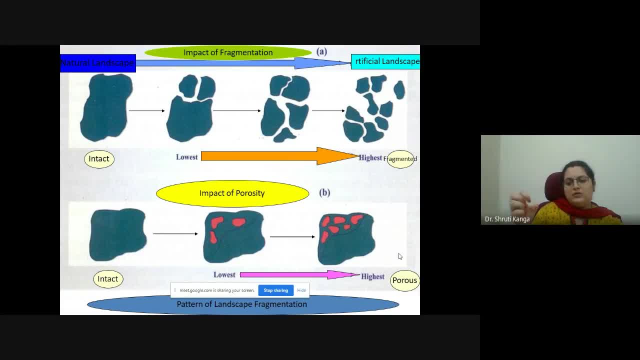 of the interference of different, you know- elements, different habitations, different activities. the forest is being depleted and slowly, slowly, it is being, you know, fragmented, Okay, Okay. So you see, these are the natural landscapes. okay, now they are the fragmented ones, they are the lowest fragmented ones. okay, when we have only two or three patch out of this land. 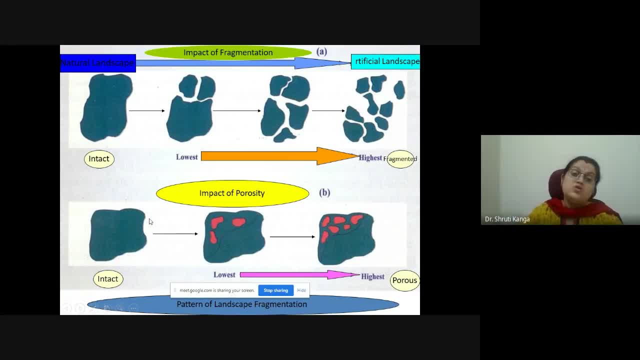 or we have only two or three patch out of this land. So in this case, the less fragmentation has been took place, but here, while it is in fact increasing with time, the more fragmentation is being taken up. It may be because of the- you know, encroachment of different habitation, different land use. 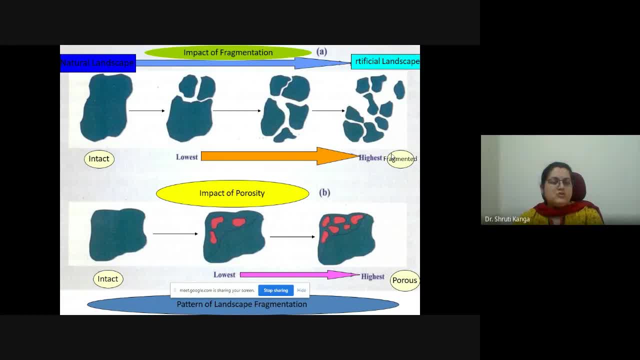 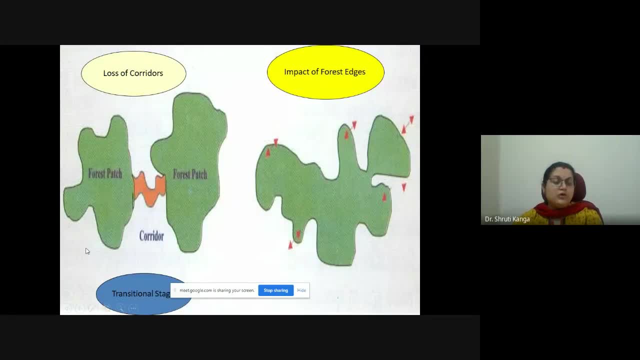 classes into the natural landscapes. Okay, That's why we have a cases of fragmentation, Then loss of corridor, obviously when we have, you know, fragmentations due to any land or land use. So that's why we have a cases of fragmentation, Then loss of corridor. 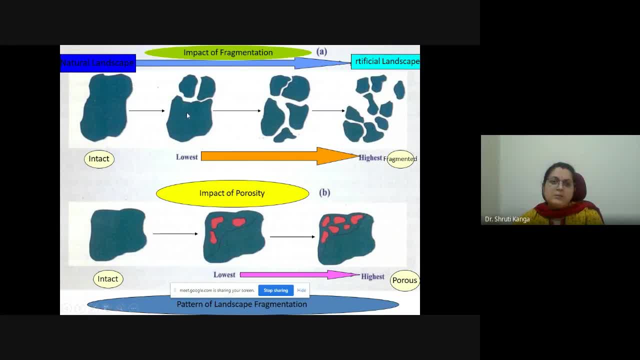 So that's why we have a cases of fragmentation, Then loss of corridor, Then loss of poured soil and what is called as the definition of fragmentation. So, in addition to the fragmentation, so after youですet a very different Natural landscape, Obviously, and without manpower, without machineries, it cannot work if we are trying to put up. 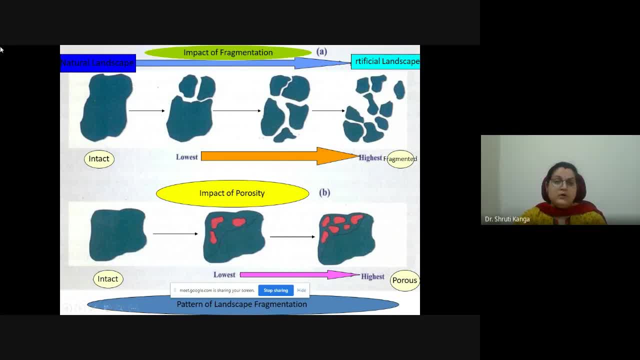 So suppose now this industry has started blooming so more manpower will come and obviously they will try to stay nearby itself. So maybe if the companies here they set up their society over here, so obviously the encroachment of the habitation is there inside this natural landscape for anything. 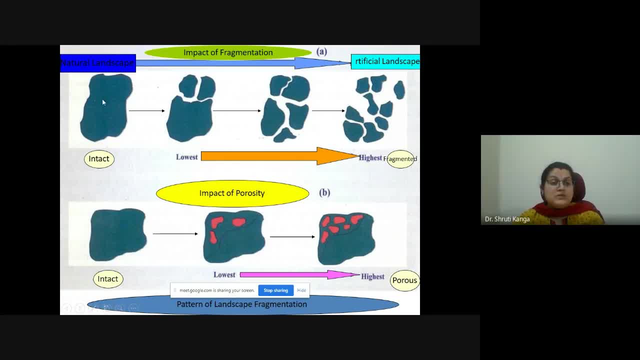 Or you may have, you know, tourism activities various. so nowadays everybody wants a place where they have tracking options, where they have scenic beauties, where they have good Amount of you know, wildlife, sanctuaries or natural parks. 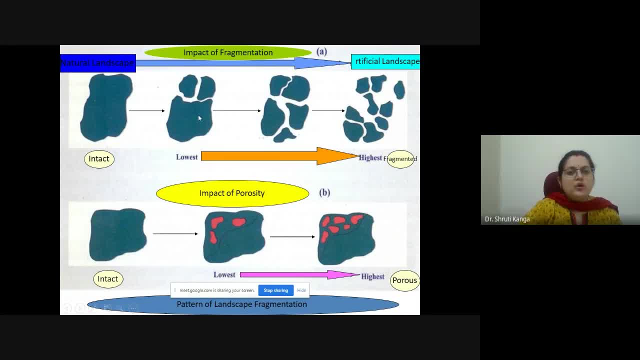 So, obviously, if tourism is there- small, small, you know different restaurants, different hotels- they will like to stay back here Inside this and slowly, slowly, these will the fragmentation, which was only one in maybe 1991, it will be, you know, 10 in numbers in 2001.. 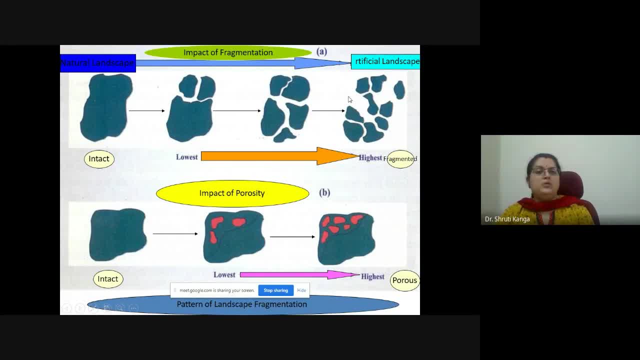 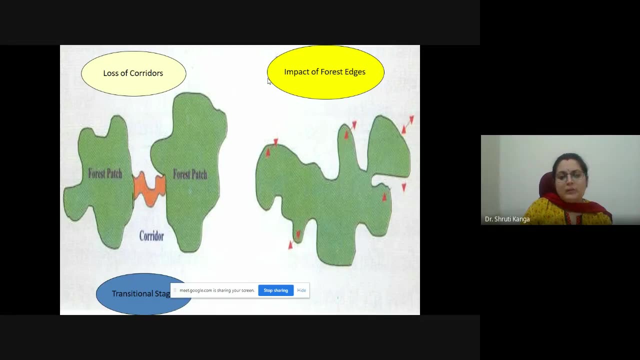 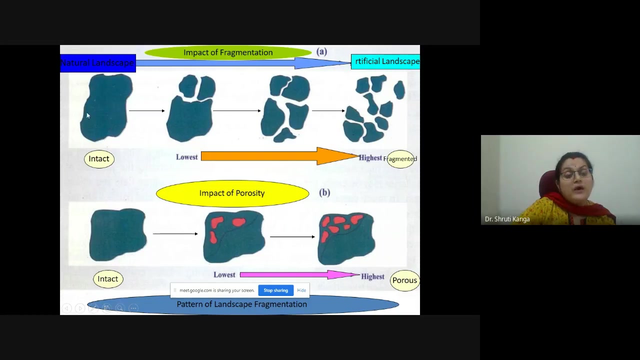 And it will. It will be 20 numbers in 2020.. So this is the impact of fragmentation. If there is one fragmentation, maybe with time it will increase, And then, obviously, if there will be a fragmentation, so there might be some wildlife sanctuary or you know wild flora and fauna who are inside. 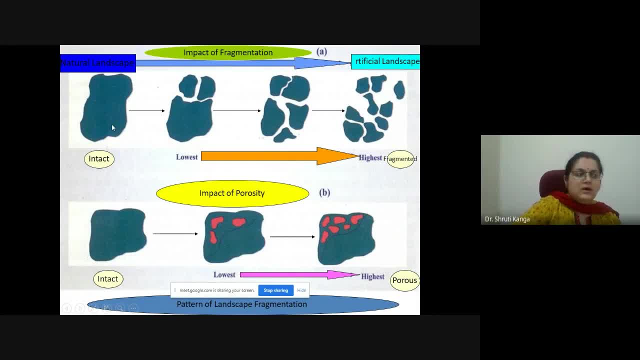 For whom this is A You know, Okay, All right, Yeah, Okay, um, acting like a shelter for them, and it is also providing them food, shelter and everything. but if these human activities, uh, due to these human activities, some encroachments are there, 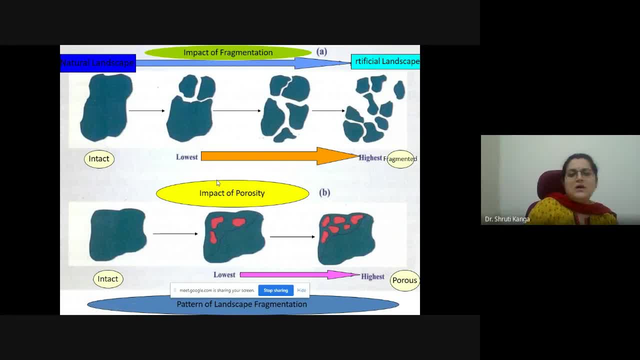 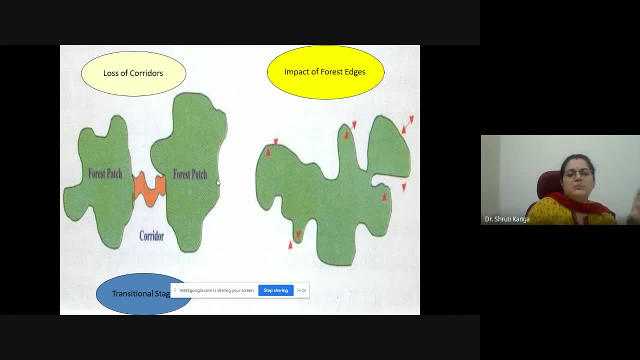 or some uh you know interferences are there. obviously, we are also, uh, you know, disturbing the life of the people uh who are uh or the habitats, or the uh you know um wildlife who are uh having their habitats inside these forested areas, and it is also, uh you know, losing the corridors also. 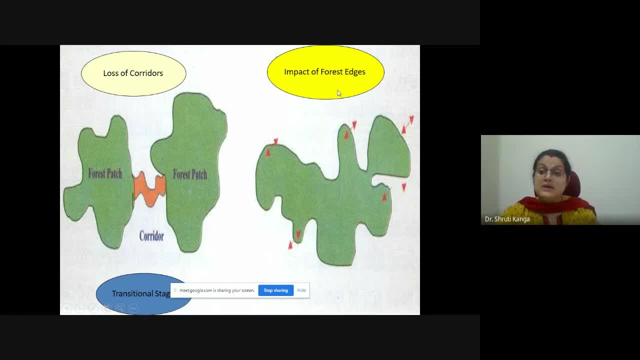 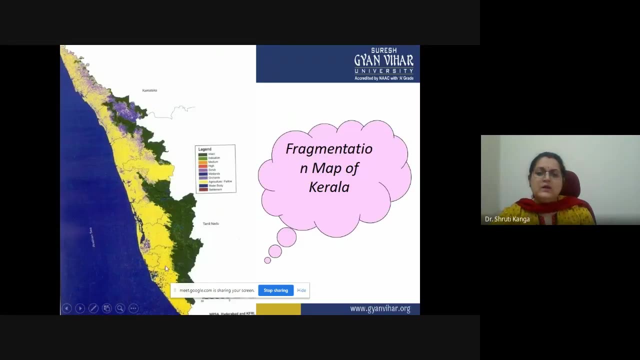 it is also impacting the forest edges. they are becoming either smaller, which are earlier broader, or maybe it is being fragmented into different, different parts. okay, then the fragmentation uh. map of kerala. if you see the different- uh you know categories are being done in this case study. 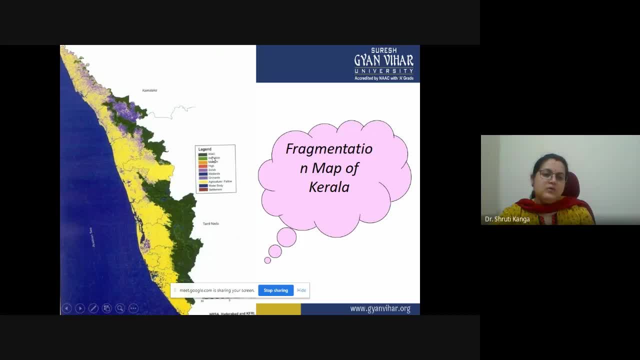 as far as the fragmentation is- uh- you know uh- concerned, so the areas which are in green, they are impacted areas, and then, uh, the wherever there is this light green- uh you know uh- areas. they are indication where these- uh you know- fragmentations are about to happen or they have started happening now this 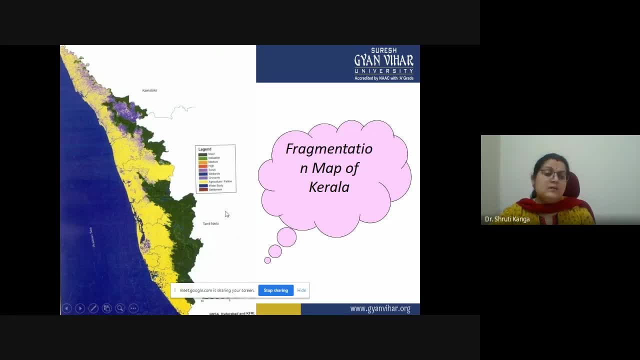 orange color, this is denoting there is a minimum- uh, you know, fragmentation. and wherever there is a red color, it is denoting the fragmentation, and then the fragmentation is going to happen, and then the fragmentation is going to happen. so we have to start noting the high fragmentation. 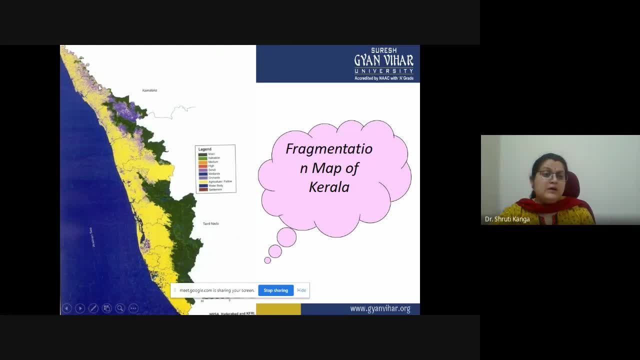 the areas in, uh, purple color, they are the scrublands. the area in dark blue color, they are the wetlands. the area in light, uh, uh, you know um this thing, um purple color, they are the orchards, the yellow is the agriculture. so now we have tried to give the fragmentation area, along with the 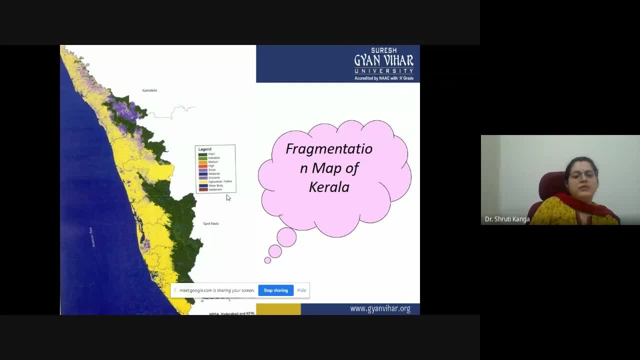 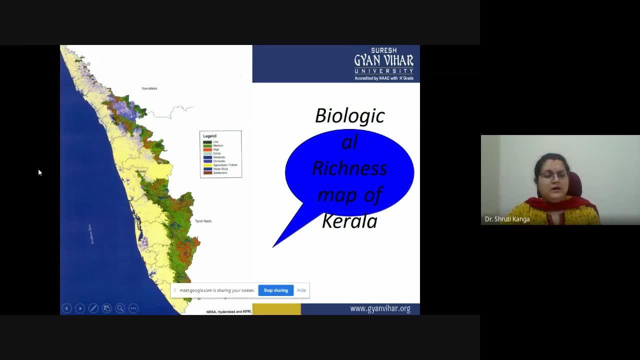 land use, first class land use in the kerala state, then the biological richness map of the kerala. if you see, uh, in this case study they have also tried to, uh, you know, uh do the biological richness map where it is very low, where it is medium and where it is high. okay, then, uh, the brown color it. 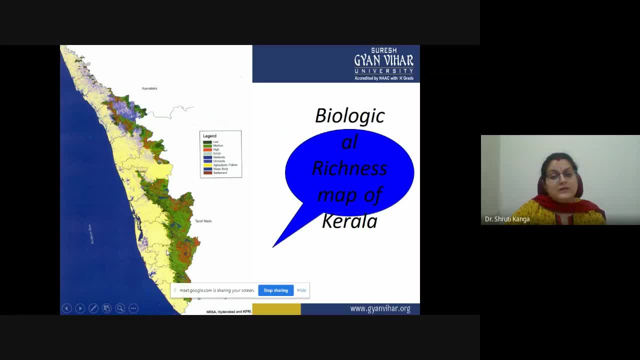 is denoting the- you know, settlement inside these areas, agriculture, orchards, so all these categories are that only. but where we have biological richness, these key areas are indicated by the red color, and where we have low richness, we have, uh, they have tried to. so this kind of uh you know, uh- calculations can also. 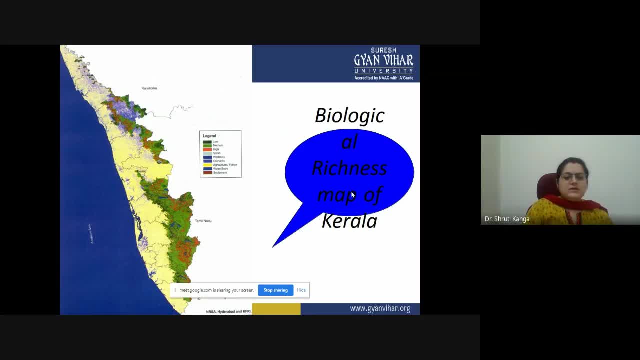 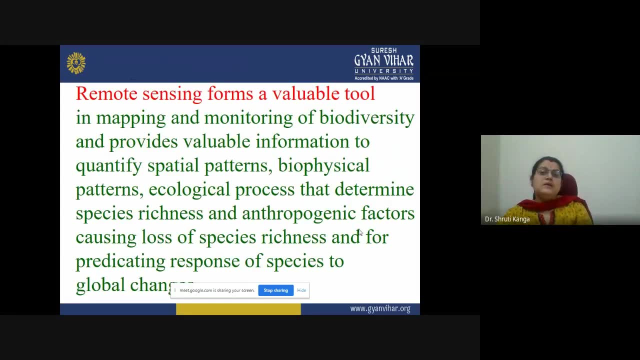 be done for the complete state with the help of these geospatial technologies. now, if you see uh this remote sensing has a valuable uh. it has acted like a valuable tool in uh the forest mapping, any kind of mapping. we why we are uh telling forest mapping? because 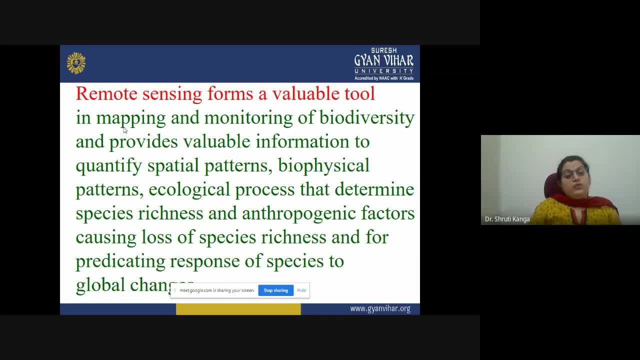 our uh concern is right now uh to for the forest mapping and monitoring of different biodiversity, and it also provides us the valuable information uh uh to quantify the spatial patterns: what spatial patterns of forest that particular area is having if you go through the different time series data. 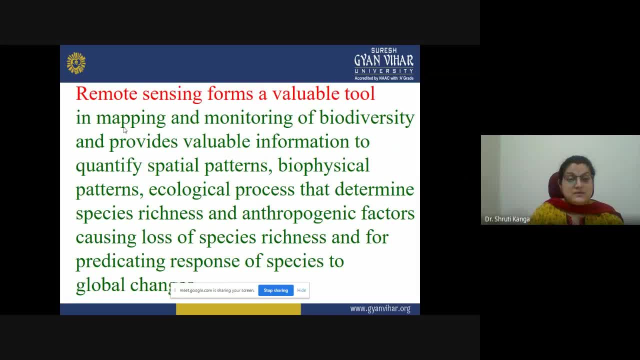 sets, but is bio physical patterns. they are following what is ecological processes that determine the richness of the- uh, you know, species and the anthropogenic factors which are causing the causing the loss of species richness, and for predicting the response of the global changes. so, remote sensing, it is a very valuable tool. as far as the mapping is concerned, I told you how. 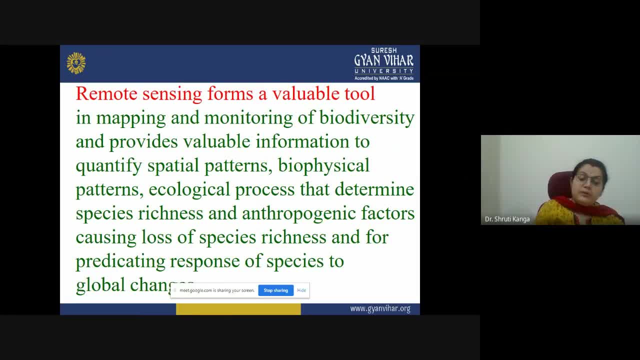 because we have a synoptic view of a complete state in a one go. we have an option: we can clip an area if we want to go for a study of individual forest division, okay. or we can monitor the biodiversity and we can also provide the information, which is very helpful, to quantify the. 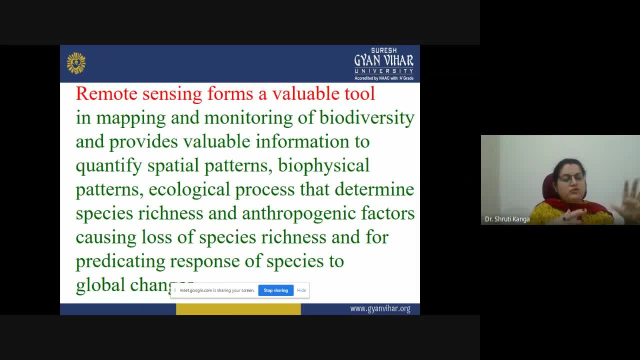 different geological or spatial patterns of the forest in a particular area? what are the different biophysical parameters? what are the ecological processes and and the anthropogenic reasons due to which the richness of different species is being hampered? okay, they may be the settlements, they may be the. 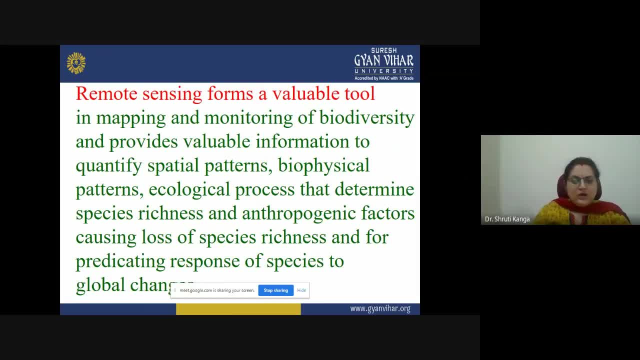 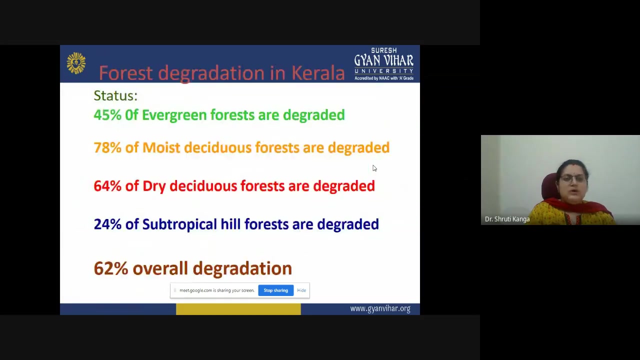 road networkings, they may be the industrialization. so all these kind of things we can do very easily with the help of these geological parameters- eu special techniques okay- and they are also helpful in predicting and analyzing the richness and the- you know, different global changes in a particular area. now, if you see the 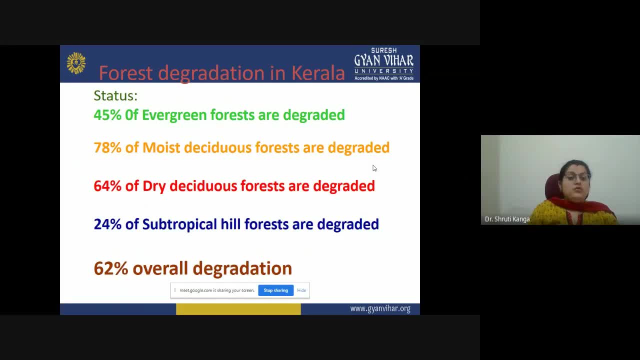 statistics or the status of, you know, forest degradation in the Kerala is 45 percent of evergreen forests are degraded. okay, 78 percent of the forest have degraded in берough hearts. but the presentation, if we keep it, a one- unprecedented. but if we come accross to these tectonic communities, if we plot the greatest number layer first in the geospatial plan, then gold processing, Istanbul, people 저기, alem of vice, phballien, go esli, are also the geospecial elites, okay, and they are also helpful in predicting and analyzing the richness and the- uh you know- different global changes in a particular area. 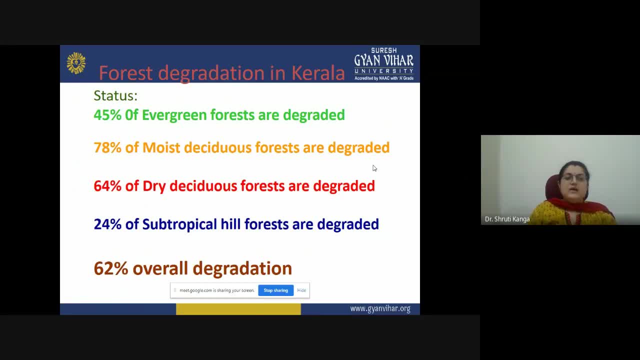 now, if you see the statistics or the status of, you know, forest degradation in the kerala is 45 percent of evergreen forests are degraded. okay, eight percent of the moist, deciduous forest is are. this is as per the case study. i have done nothing, i have just trying to show you the different- uh, you know- things which people have. 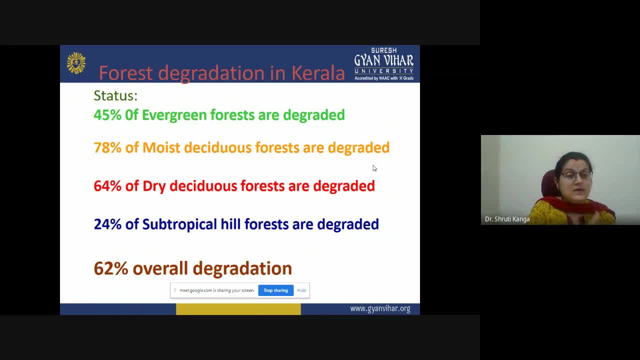 uh done it in their studies. now, all these things, with more modifications, you can also do in your uh uh, you know uh coming desertations or your uh you know uh studies. so my aim is to make you aware that what kind of things people or the scholars are doing as far as the forestry, 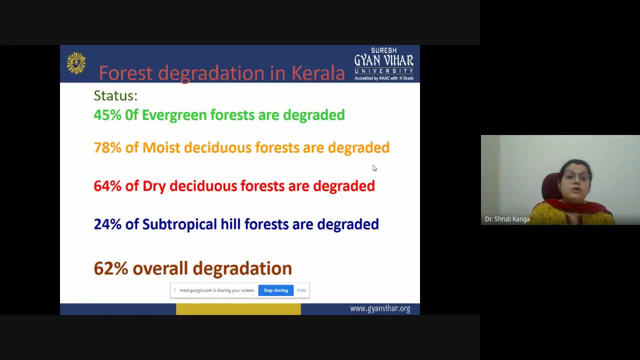 applications of these things are concerned. they are going for species characterization, they are going for biodiversity richness, they are going for carbon sequestration, okay. so uh, they are going for the forest degradation as per the temporal basis. so a general status. so uh, there is a loss of 45 percent of evergreen forest, 78 percent of moist, deciduous forests. 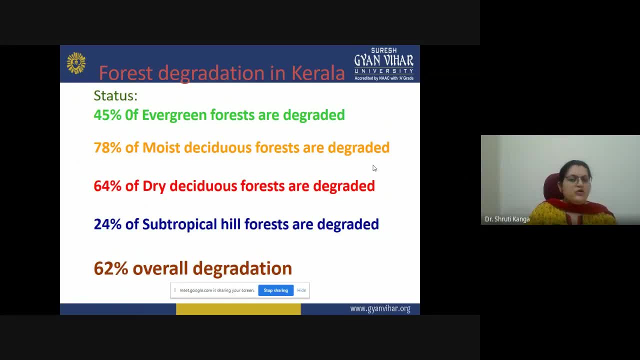 are degraded. 64 percent of dry, deciduous forests are also degraded. so, uh, you know type wise. different forest categories have been impacted, different as far as their- you know- degradation is concerned. so, overall, different degradation. if you average it, the overall degradation which took place as far as the forest degradation is concerned is around 62. 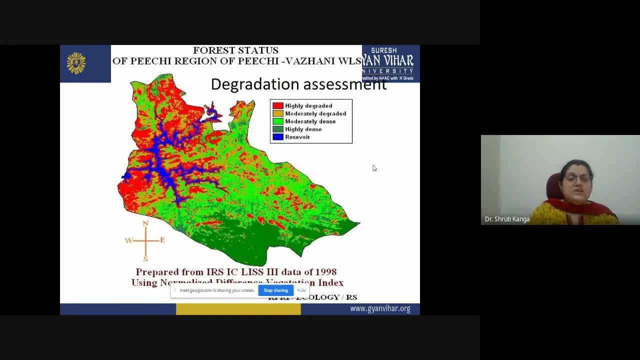 then the forest status of peachy region of, uh you know, uh, the karela. so is the the uh, the uh. this is actually, you see, the drainage assessment. they have done so they may have taken various parameter and they have gone through the different overlay analysis of those, uh you know, um layers and 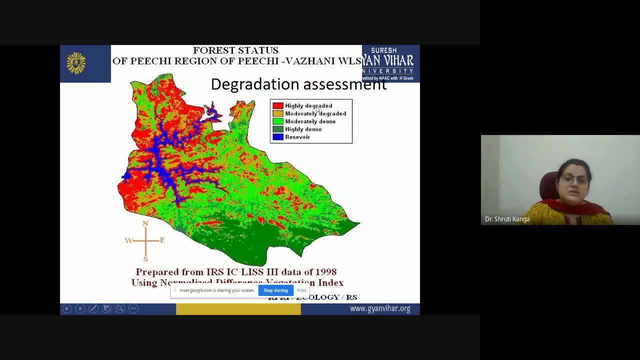 then they have calculated the degradation assessment on the basis of their severity. so the areas which are in red, uh, they have, they are highly uh degraded. and then these areas in the yellow, they are moderately uh. the areas in parrot green color, they are moderately dense, highly dense, and reservoirs. so you see, uh, in the north and the western part there is a maximum. 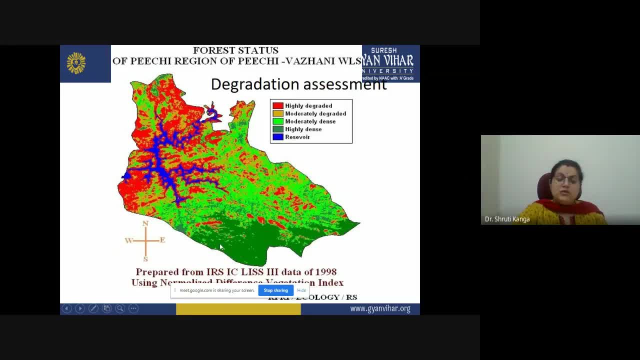 uh degradation which took place. so they, for these studies, they have used this three data set and they have done it with the help of ndvi, that is called as natural normalized differential index, in which we take into the infrared and red bands into consideration. and uh. then 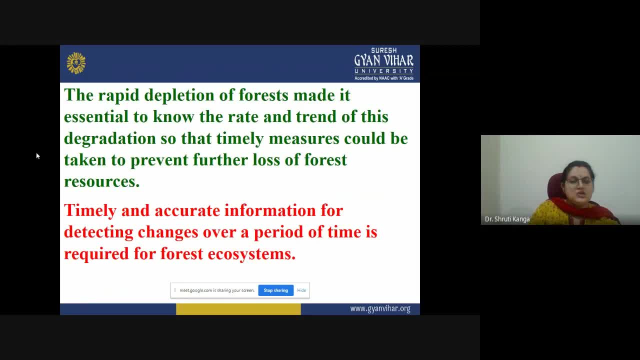 the rapid depletion of forest made it essential to know the rate and the trend of degradation so that the timely measures could be taken to prevent further loss of the forest resources. okay, so, uh, the these, these techniques, they are helpful in the rapid uh depletion of the forest: identification and based if, if you, if we know that which are the areas which are. 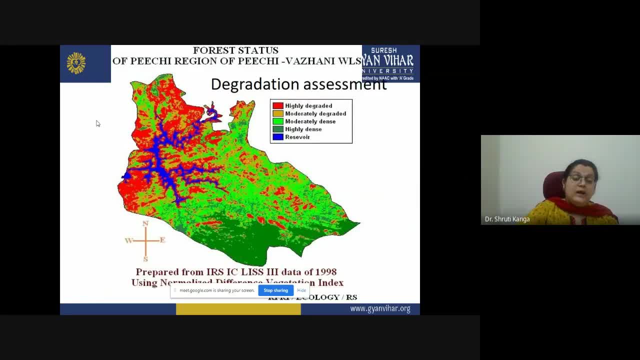 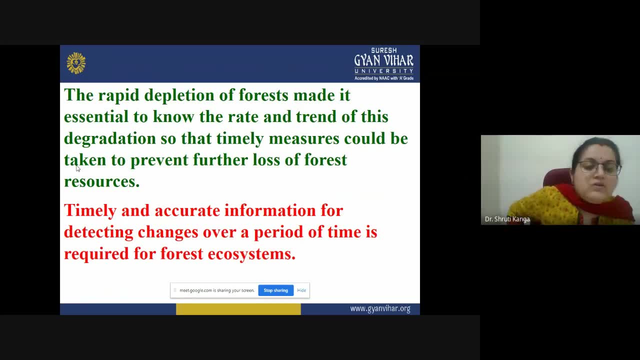 having high and moderately high and no loss as far as the degradation is concerned. so it is easy to go for different kinds of preventive measure for the uh different forest department, for the different uh people who are working for the uh, you know, sustainable management of these forests, then timely and accurate information for detecting. 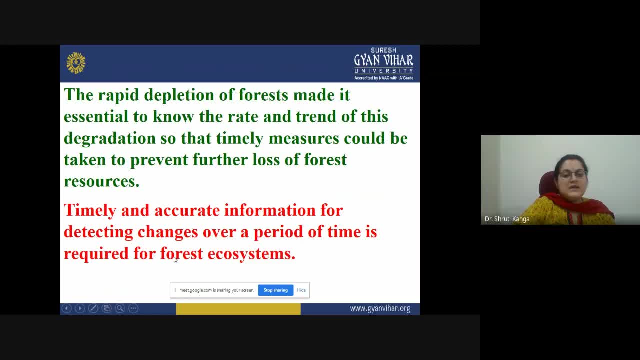 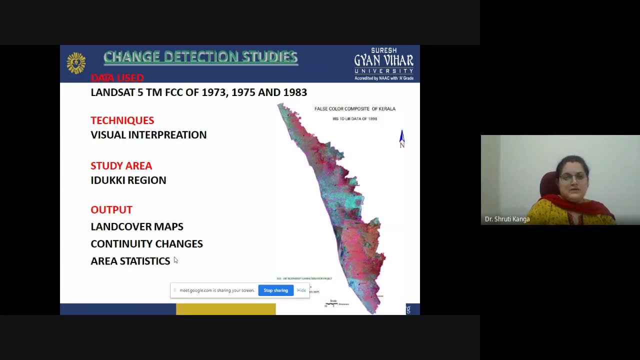 changes over a period of time required for forest ecosystem and what kind of you know- plannings can be done on the basis of- uh, you know, different time periods. that also can be decided with the help of these kind of things. then the change detection studies were also done. 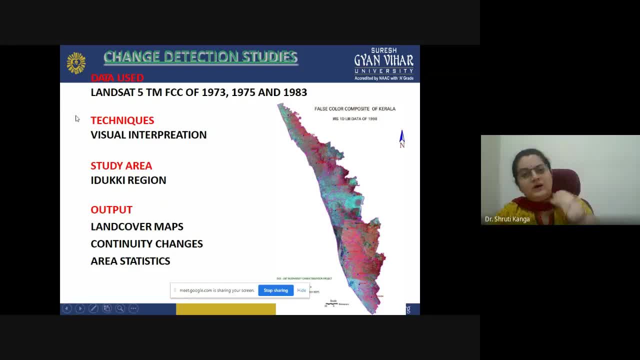 where, in this case studies, they have used uh, the landsat thematic data set of 1973, 75, 83, so different time periods, data they have taken. then visual interpretations were done and the study area was a ducky region of karela. the output was in the form of land use, land cover. 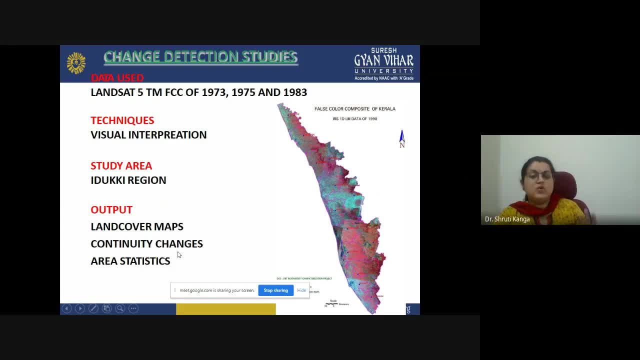 map, continuity in the changes and the area statistics. so you with the use of different models, okay, uh, in this case, studies. they have tried to know about the land use, land cover in that particular area and based on the aerial statistics. they have also gone through the aerial statistics. 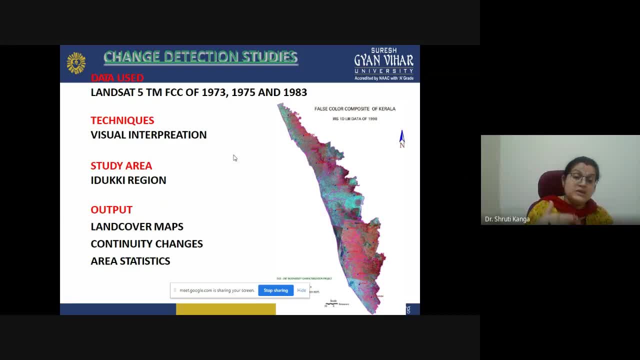 that each land use land cover class has how much area under a particular class for different years. so if you go through and compare these uh area calculation, uh year wise, then you will come to know about the land use land cover change in the study area. okay, so 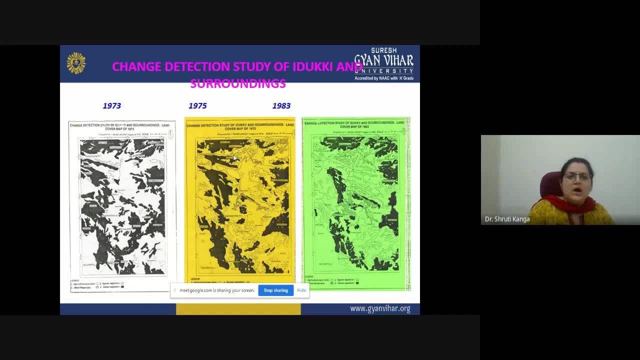 these are the images which they have used and these are the uh change detection in and around the study area. so you see this area. if you see this, this forest, okay, this is this much in 1973, whereas if you see this, this area, this has converted into some other area. okay, so that means this area has reduced this forest. 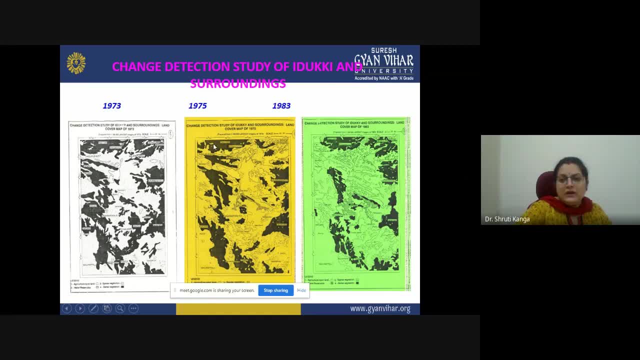 area is reduced and if you see here, from 80, uh, 75 to 83, now this, this forest area is also converted in some other land use class. now here we have so much of forest. it has reduced in 1975. if you see in 83 it has reduced much more. okay. so these kind of change detection related studies in terms of 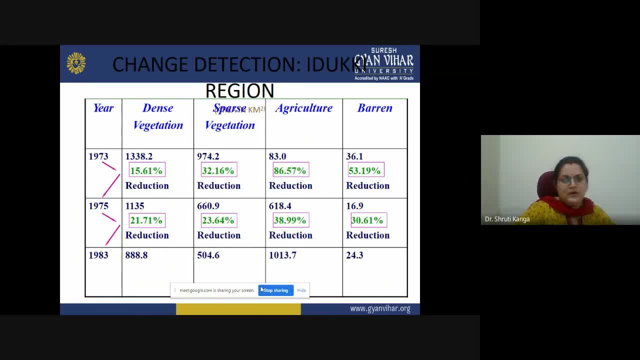 their aerial calculation. we can go for: okay, you see here, in 1976 the dense forest was 15.61. okay. in 1975 it is reduced up to 31, point this percent. okay. and in 80, uh, uh, you know, in 1983 it was only 8.8, 88.8 square kilometers. okay, you see. 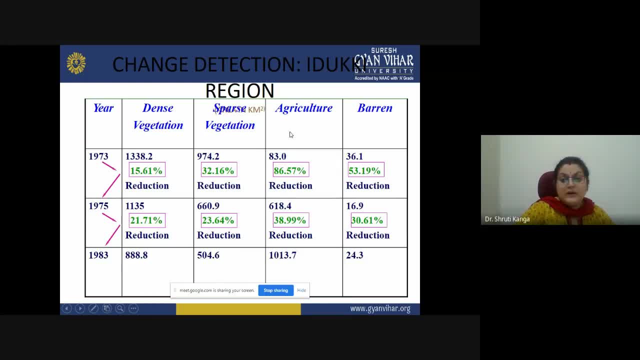 everywhere there is a decrease, okay, but in agriculture it has increased, so maybe this dense vegetation or sparse vegetation land has been converted into this category of land. okay, now, barren land is also more discrepant than bare land, and now we are talking about So the land is almostуб там. we have to someday go for this plate, and this is the name of beach. 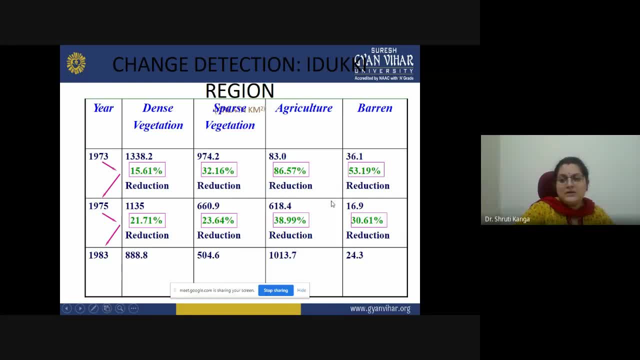 you know it has decreased here but it has again increased here in 83. but if you see, this is our mean, this thing. so the land use, land cover has been changed, so landscape has been changed from maybe dense forest to some extent to agriculture activities. yeah, then we have this change detection. 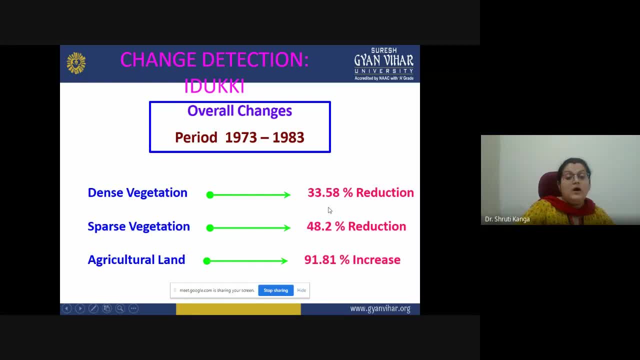 dense vegetation has reduced up to thirty three point five, eight percent. if you compare, or if you have, if you calculate, from 1972 to 83, in just ten years it has reduced up to 33 percent the sparse vegetation, what it was earlier. it has used up to forty eight point two percent. this is as 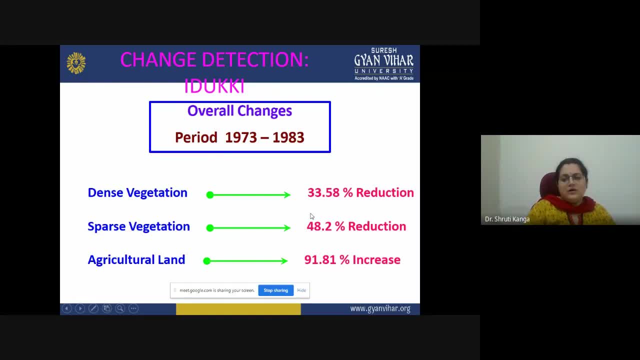 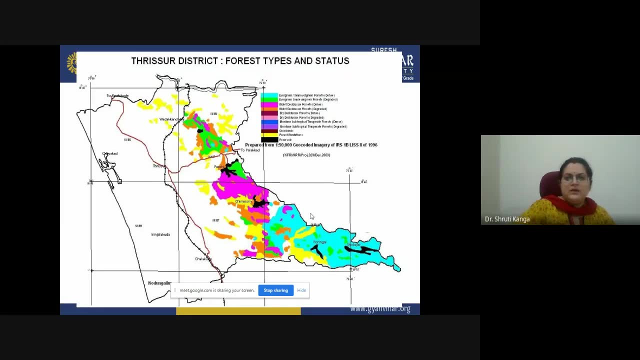 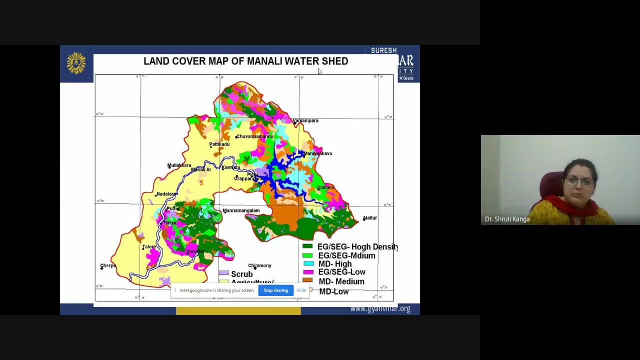 per the case study, and they must have some, you know, calculations done with reference to the quantification activities in the area. okay, now this is a forest type status in some other part of the same state. this is land use. land cover. map of sorry watershed. map of the Manali. 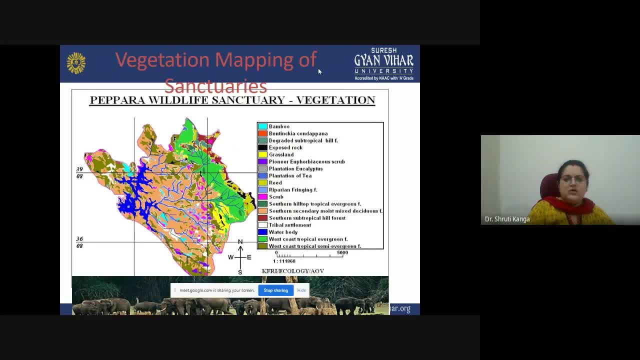 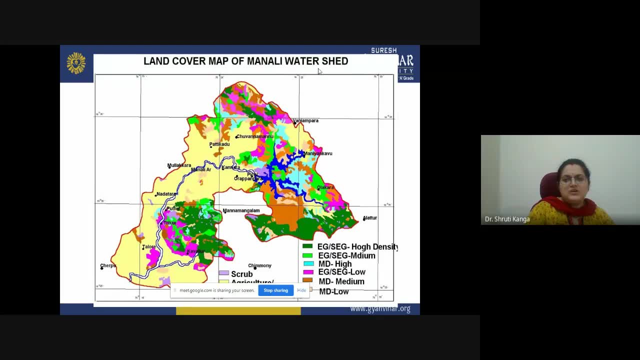 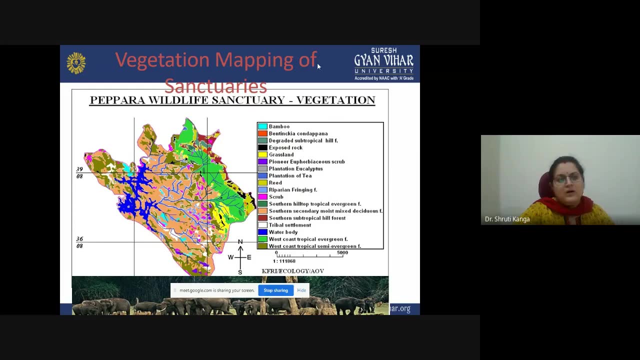 watershed of the area so we can also go for the watershed delineation and what are the different quantification in that particular area that we can also go for? then the vegetation mapping in this uh papara wildlife sanctuary. okay, so we have uh these many forest types uh here in this wildlife. 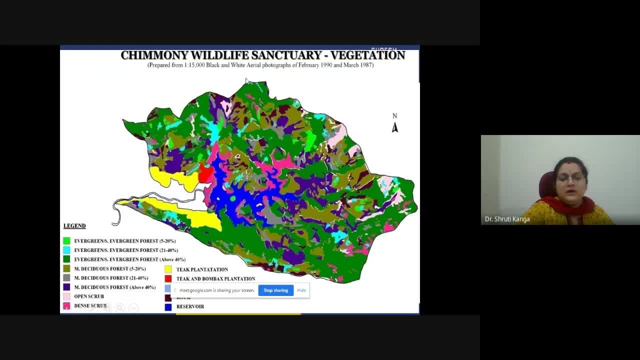 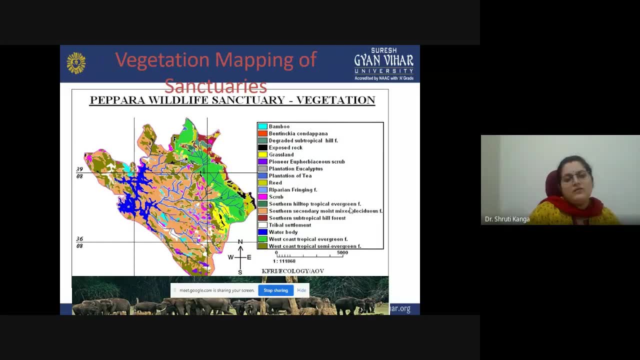 sanctuary, then the again one more wildlife sanctuary. so in this case study, they have tried to. you know, a forest we can cover. we have seen that they have gone through a vegetation mapping. they have gone to a wildlife sanctuary vegetation mapping. okay, on the basis of this we can decide. 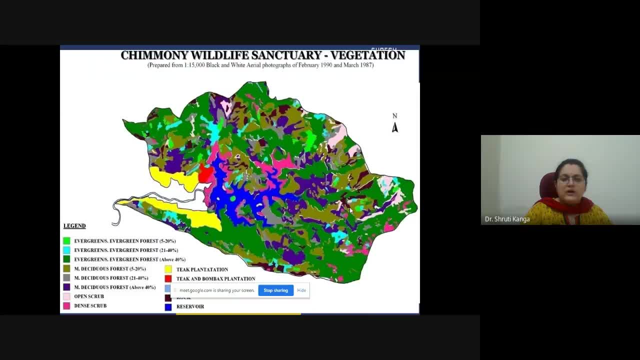 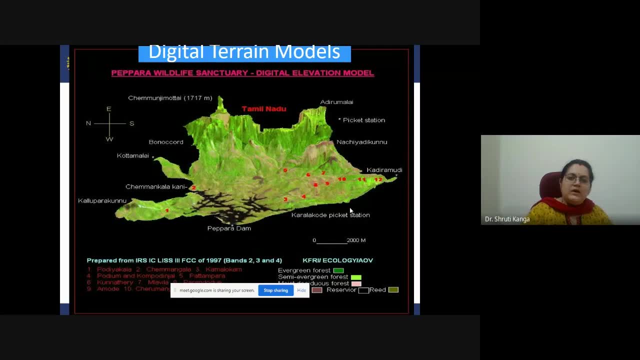 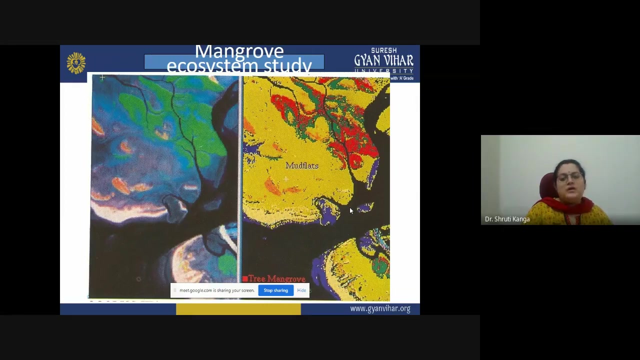 key. what kind of activities can be done or what kind of wildlife is there inside these sanctuaries? okay, then we have the Terran model. we can have an idea about the uh topography of a particular area based on these analysis. okay then the mangrove ecosystem study also being conducted for the 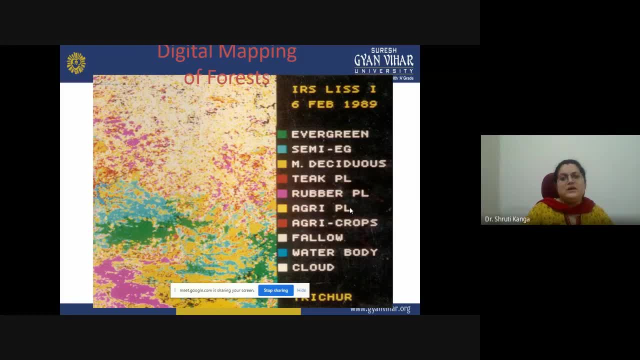 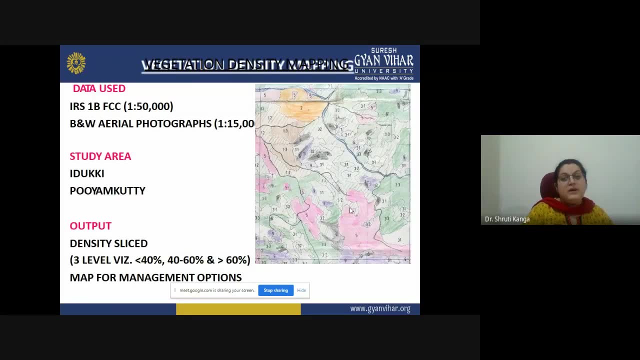 same area, the digital mapping of Forest can also be done with the help of these kind of studies. then the vegetation density mapping, where they have used uh, you know NDVI technique, and the density was sliced on the basis of different three levels: where we have the classification with where we have uh calculated, uh below 40 percent maybe. 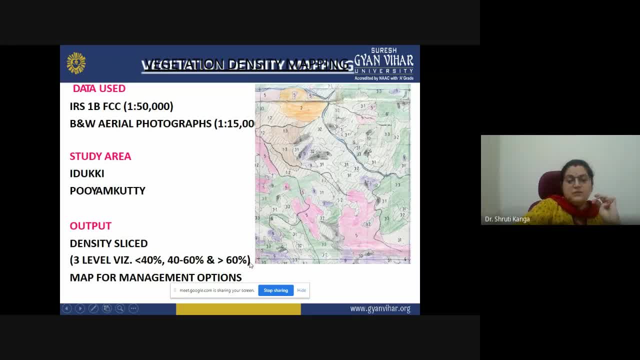 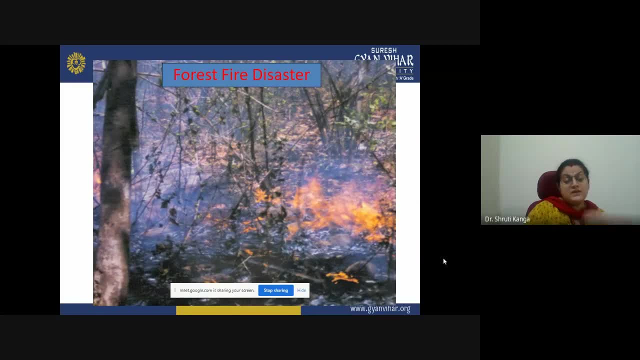 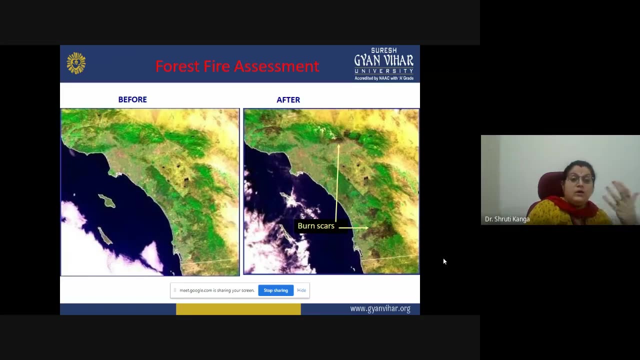 degraded Forest: 40 to 60 may be dense and more than 60 maybe, uh, the very dense Forest. okay, then the forest fire disaster was also found in the area. okay, then, forest fire mapping uh of before and after fire. now, after fire, you can see the scars on the forested areas. okay, so this is the image where 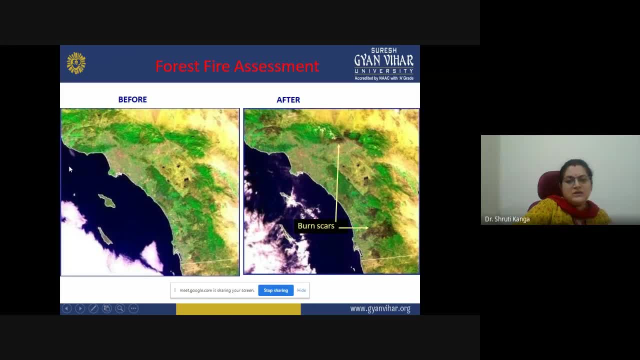 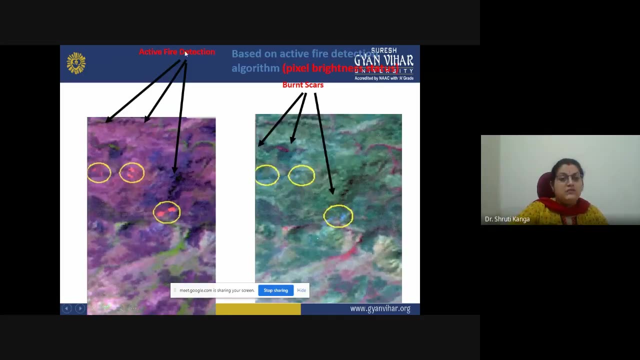 you can see the before situation. it is a clear cut Forest, but here, after the forest fire, you can see some patches of, you know, fume after fire activities. okay then, uh fire, uh, active fire detection can also be done, uh, based on uh, some uh data sets of modis or something like that. then this kind of images can be seen when we go for the. 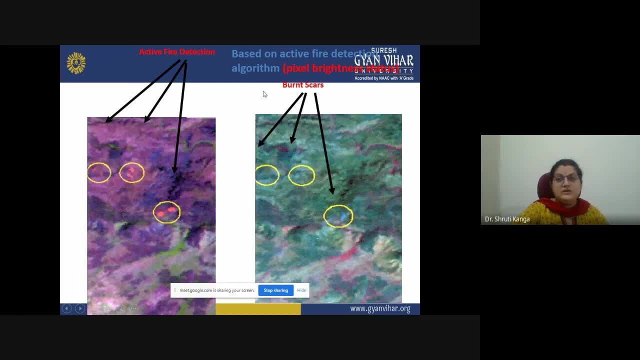 active fire detection, uh activities. okay, so pixel wise, uh you know, uh brightness values. on the basis of that, we can also go for the analysis of burnt area scars, see how much area was there under the uh burn on the basis of pixel value, uh brightness detection, obviously wherever there is a burn. 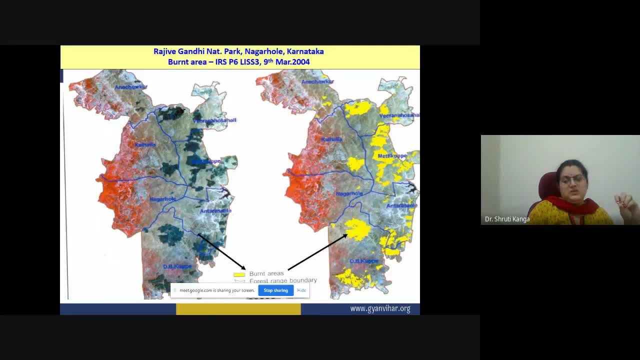 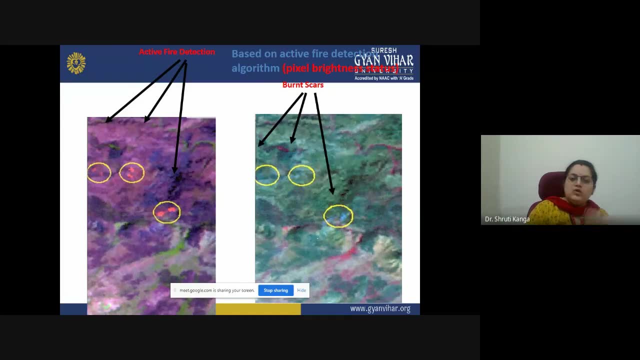 activities to place, there will be a brighter patches of, you know, pixel values. so based on that, we can identify and we can also quantify in the field that, yes, whether the scars which we are uh interpreting on the basis of the brightness status that they are uh forest fire. 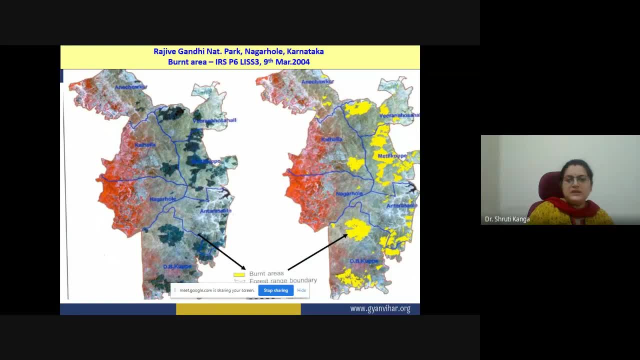 burn scars. is it so, so we can check it by going to the ground then? uh, this is a burnt area. analysis was done on the basis of: uh, you know different forest fire? uh, demarcation in Rajiv Gandhi National Park, Karnataka also. so this is the image where they have tried to demarcate these burnt areas. 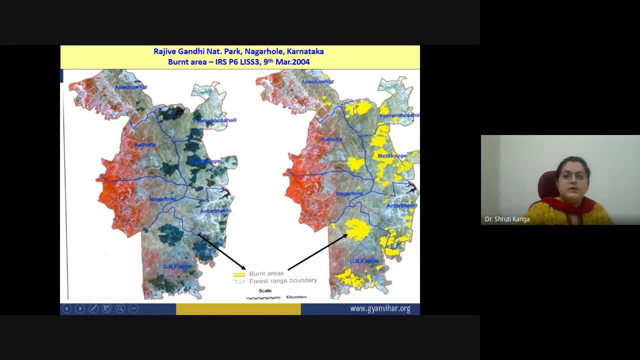 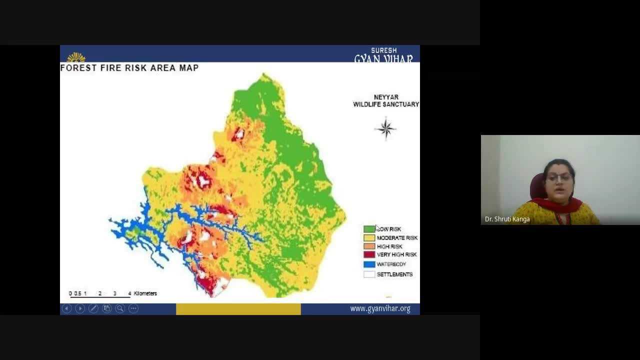 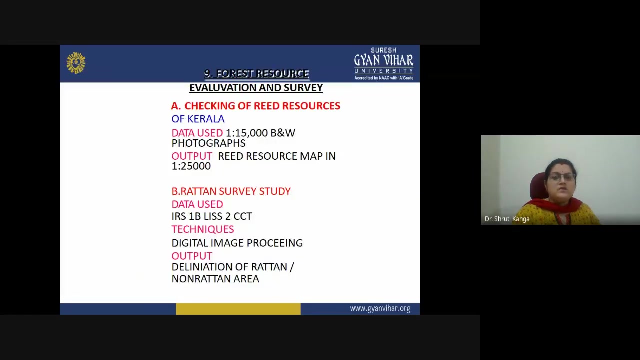 which you can easily identify in these uh images also. then this is a forest fire risk map where they have tried to categorize the various classes of uh, you know, risk of fire, uh, forest fire incidents in a particular area. then the forest resource evaluation. we can also go for the forest resource evaluation and surveys where the checking 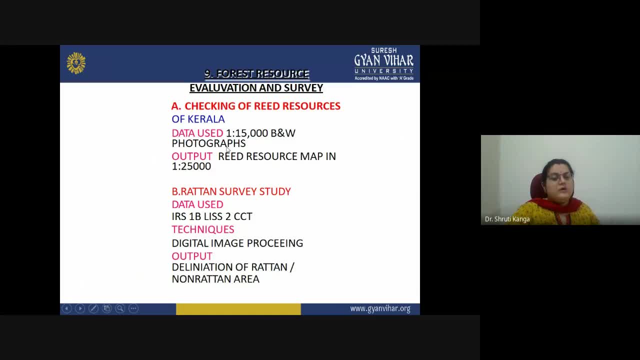 read resources of Kerala was done on the basis of, uh you know different, uh images or photographs of 1 is to 50 000. maybe on the aerial photographs, read resource map of 1 is to 25 000. and then, uh, the study area, the Ratan survey, study the data used, and these are the you know things they have. 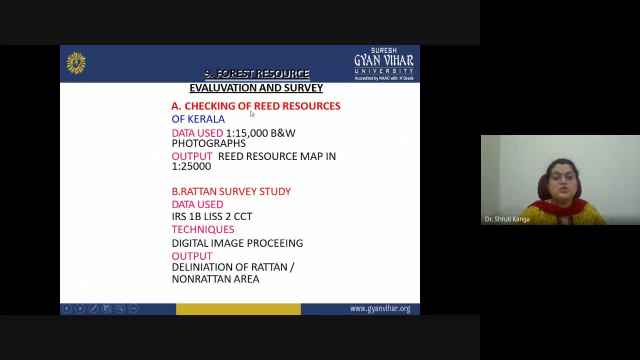 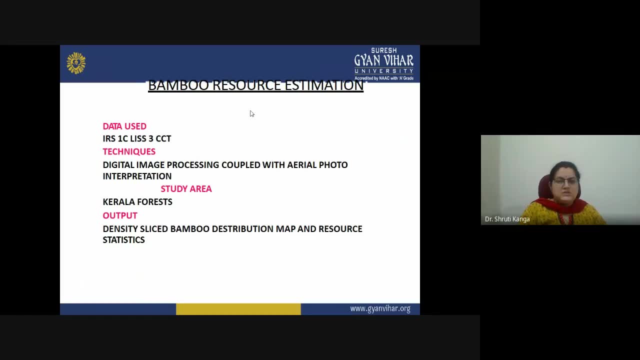 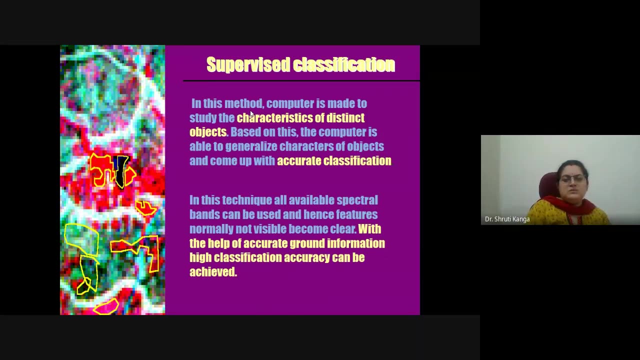 taken into consideration for forest read resources of Kerala. then the bamboo resource estimation was also done using the satellite images. okay then, uh, the they have used the you know a classification method that is supervised classification, which you have studied, uh, in your dip also, that there are two classification. 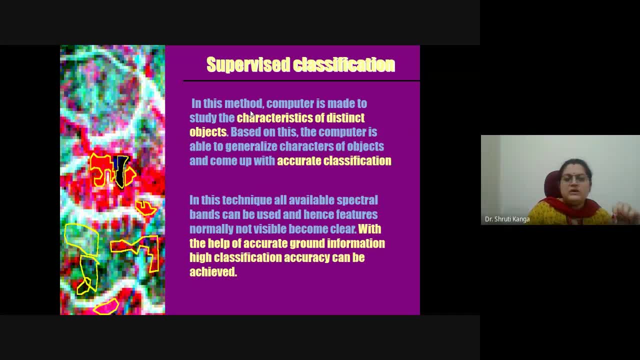 techniques: one in which we select the training sets and, based on these training set, we try to classify the whole image, and the other one that is unsupervised classification, where we assign number of classes and then we identify based on the some data sets which are being provided to us. so, with the help of supervised, they try to categorize. 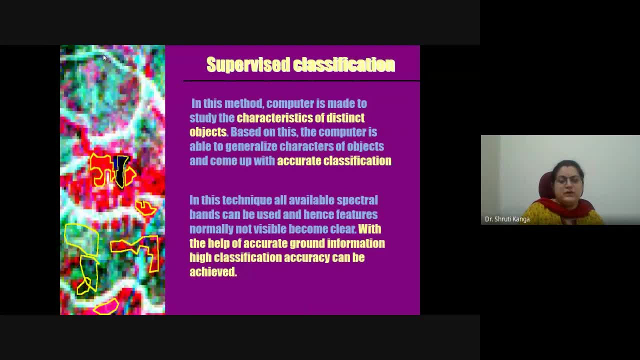 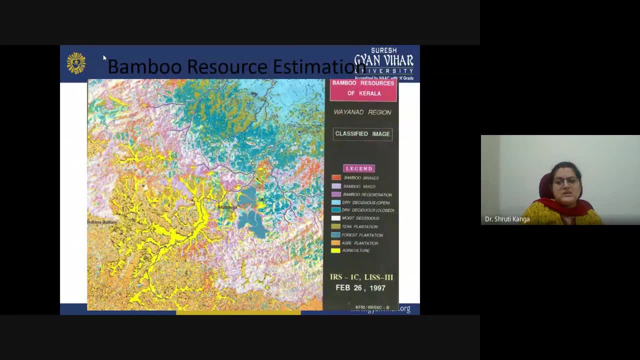 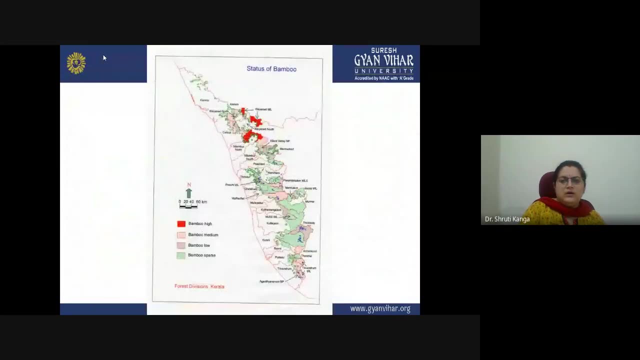 the bamboo resource estimations in the area. okay, so this is a map where they have come out with the bamboo beds and bamboo mix forest and bamboo regeneration also. okay then, uh, the status of bamboo in Kerala. here in the north, or, you know, in northeastern part of Kerala, you can find there is a high, uh you know, potential of uh bamboo, whereas 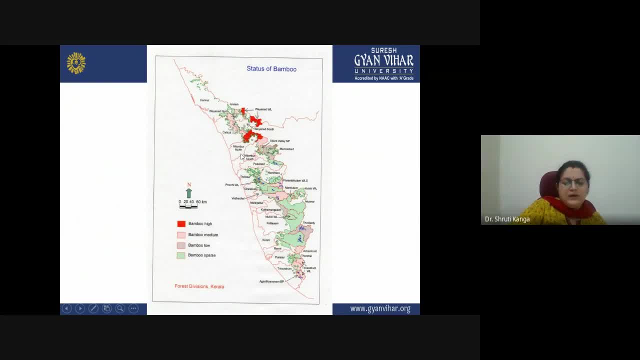 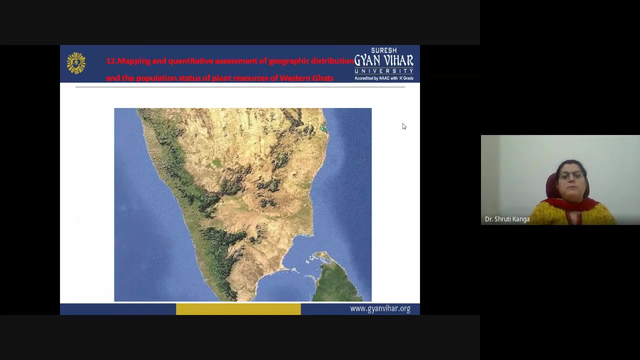 in pink they have medium potential and the area uh, you know, in uh light purple color, this has the low potential and the area in green that is having the sparse bamboo uh distribution. so this is about the uh that is also being done in by by the competitive authorities now mapping the uh. 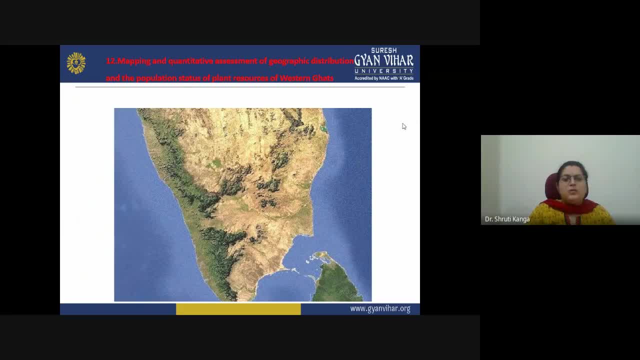 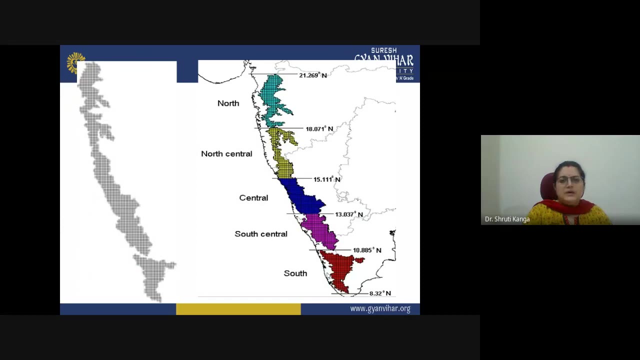 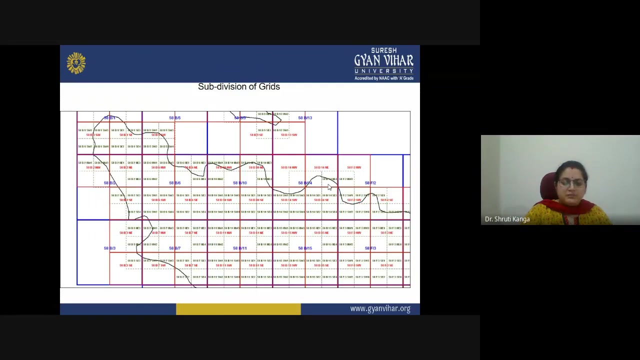 quantitative assessment of geographic distribution, population status of plant resources in the Western card. okay, so, in Western card, the population status of the plants. that is also being done with the help of different uh mapping and remote sensing data sets. so, uh, this is the things done. these are the different uh subdivision level Maps which for 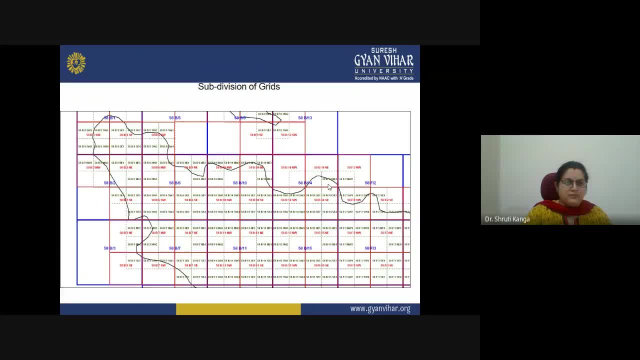 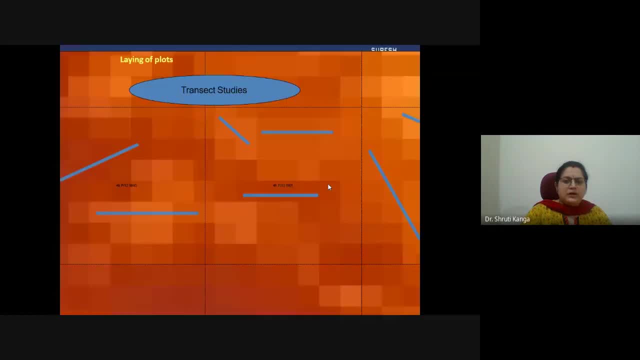 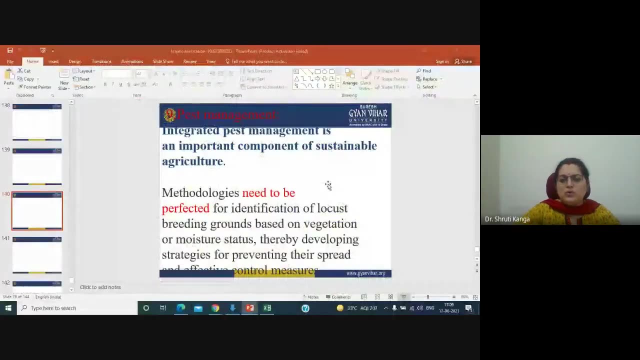 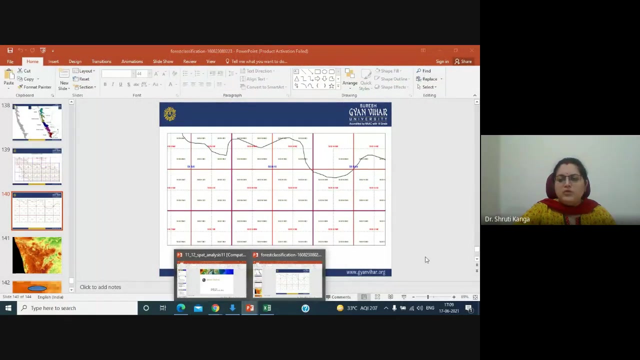 which they have used different uh sheets. this is a record of that. okay, then, different uh area density statistics also being done. so this is uh the main aim of showing you this. uh you know, uh case study is to uh become you familiar with the things. uh that, what kind of studies various organizations are doing as far as 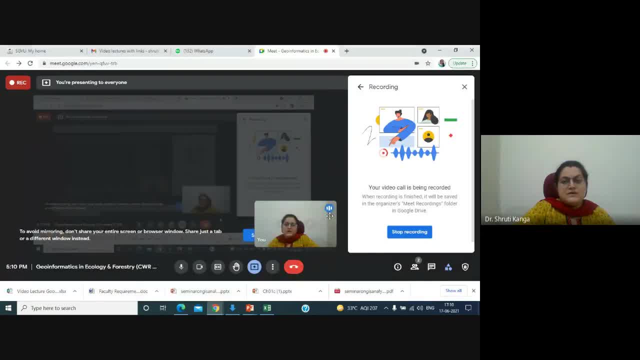 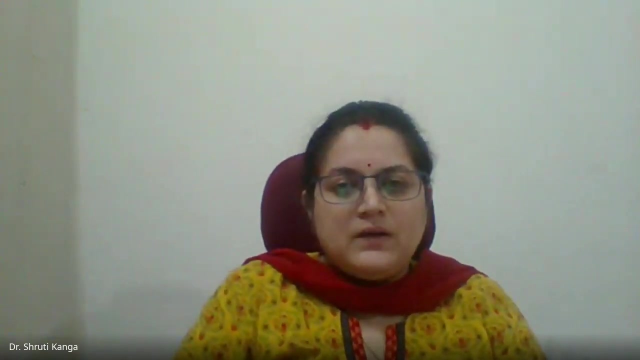 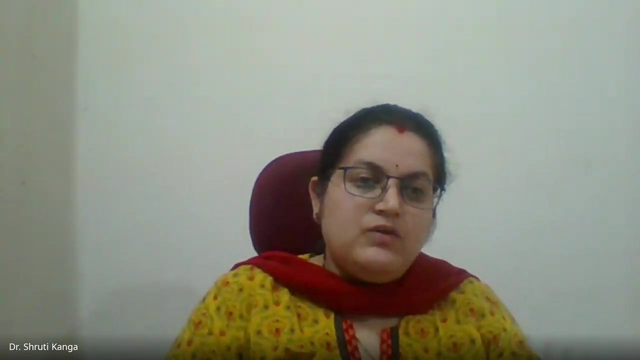 the uh forest applications of gis are concerned with reference to forestry. so with this I would like to conclude my talk. where uh we have, you know, done uh these uh forest types as per the classification of uh Champion and state. then we have also studied various uh vegetation and forestry related applications and we have also taken a case study.